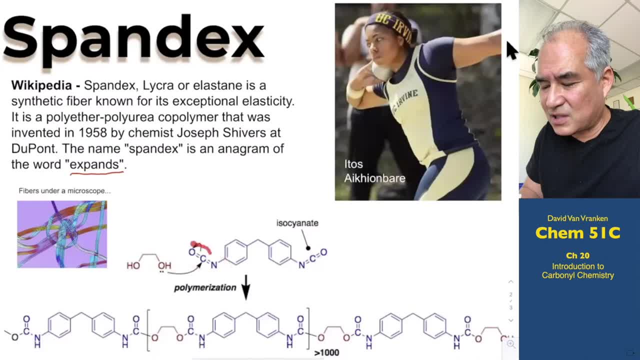 And this weird functional group that you've never seen before. this isocyanate has a really reactive carbonyl group. So alcohols or water you would Keep water out of- this reaction will easily add to the isocyanate. 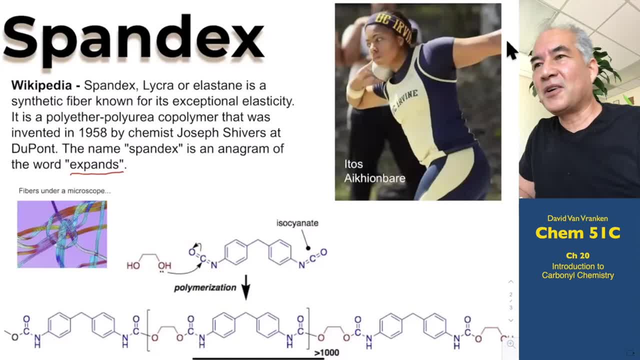 And if your alcohol has two OH groups on different ends of the molecule and your isocyanate has two different isocyanate groups, then after one alcohol adds to an isocyanate to form a functional group called a carbamate. that I don't think you've ever seen before. 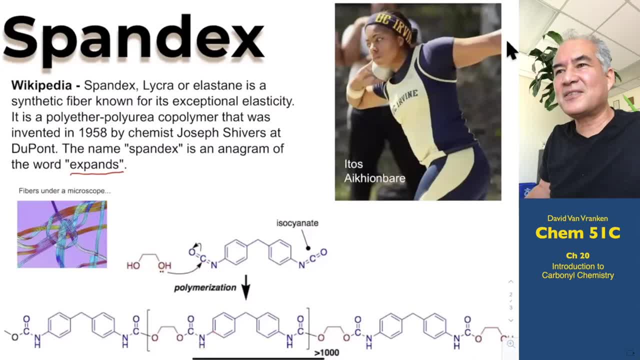 This is a carbamate. It's not an amide, It's not an ester. It's called a carbamate And it can keep reacting on each side of the molecule to make these polymers that are thousands, And that's the chemical structure of spandex. 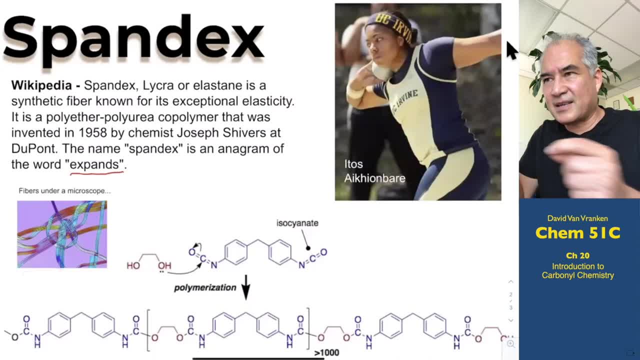 Here's a micrograph showing the strands of spandex under polarizing light, which creates those different colors, And so you wear spandex. Spandex is noted for its elasticity, its ability to stretch, And so you see it a lot in sports performance clothing where maybe, as you move your arms or your body, you want things to be freely flexible and not feel boundless. 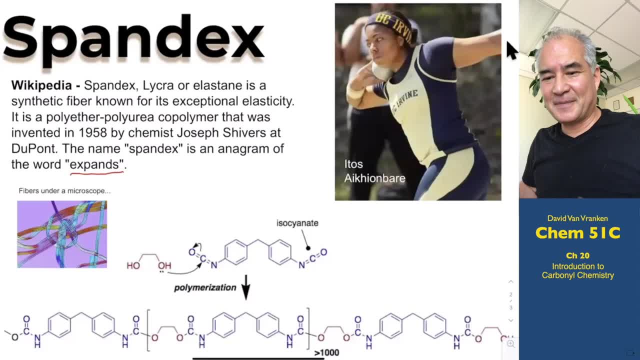 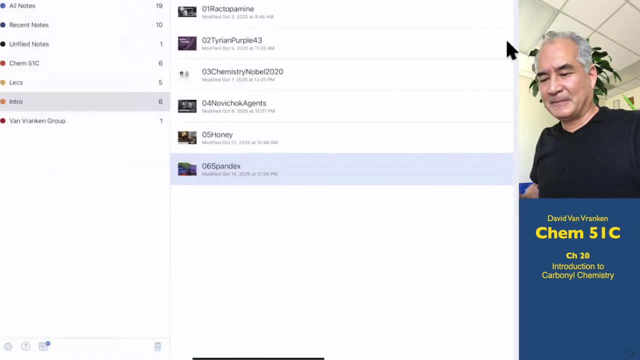 So that's spandex, That's lycra. So if you have any clothes now, you know a little bit more about the chemical structure of the clothing that you're wearing. Let's come back over and take a look at our lecture for today. 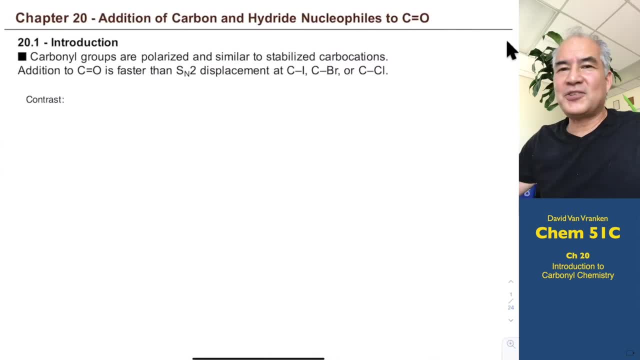 This is the most important chapter in the book And I mentioned just before we started that you know we have an exam coming up on Monday that covers electrolytes, electrophilic aromatic substitution and the acidity of OH compounds, But really this chapter. 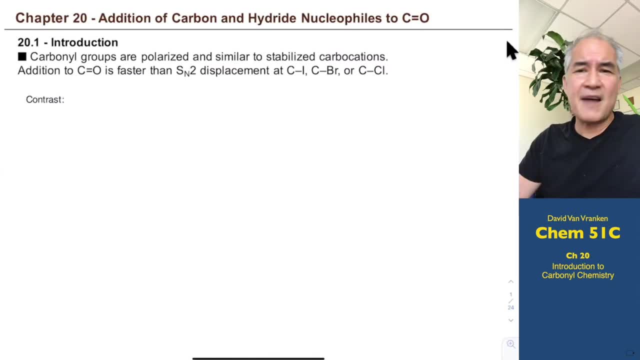 is really. it's a demarcation point between everything else you've learned in organic chemistry and the important stuff in organic chemistry, which is basically the rest of the quarter really for the most part, And so it's going to require a seismic shift in your 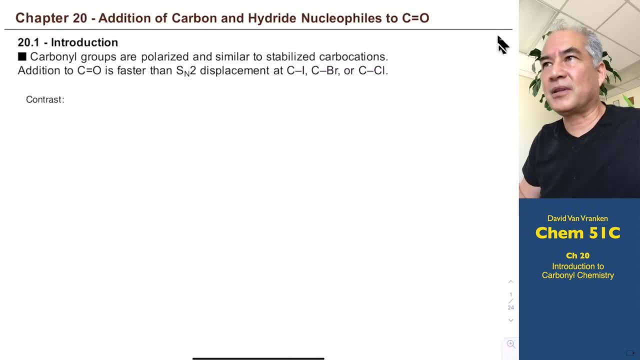 thinking. So your tendency will be to think. it's natural to think that I can't learn anything new right now. I just have to get ready for Monday's exam. But you've got to absorb this material. This is super important, And if you get off on the wrong foot here and don't absorb this material, 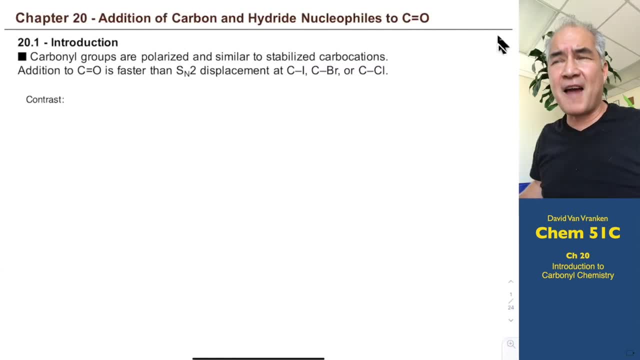 and really embrace this idea that we're going to add nucleophiles to every carbonyl that we see, then you're going to be lost. So let's go ahead and talk about that. Carbonyls- My God, that's awesome. I'm so glad that we have finally finally hit the chapter in addition to carbonyl. 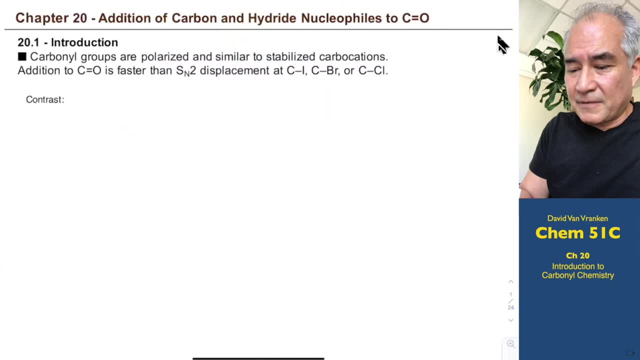 group. So I want you to contrast two different types of potential reactive functional groups. I'm going to use ET here to represent an ethyl group, Just a little easier on the eyes, I think, than writing the molecular formula. And let's just imagine that I compare that. 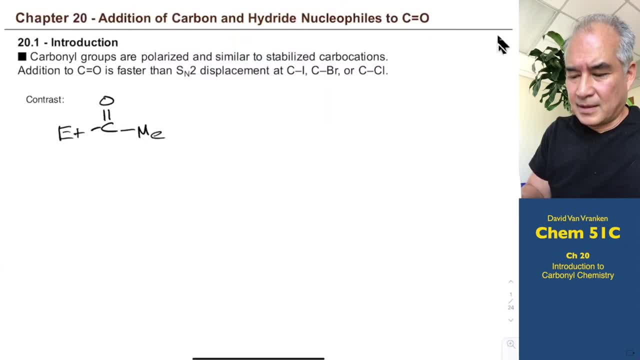 with another type of electrophile that you may be familiar with, And that would be something where you can see an obvious leaving group there, like a bromide or a chloride or a tosylate, And what we're going to do, what you ought to be familiar with, is this idea that, if you have 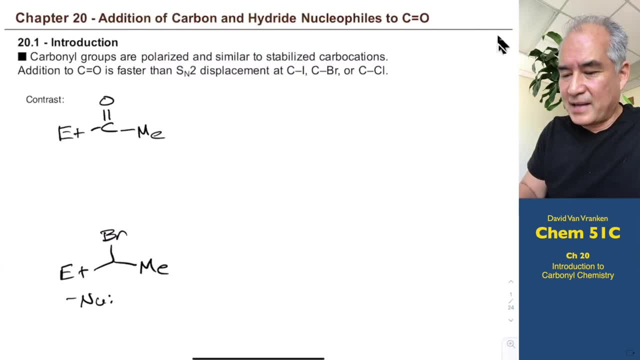 nucleophiles, then in theory you ought to be able to do SN2 type reactions and displace leaving groups. But that's really not how biology works. That's not how organic synthesis works. Why did they waste so much time trying to teach you about this idea that you can displace functional groups? 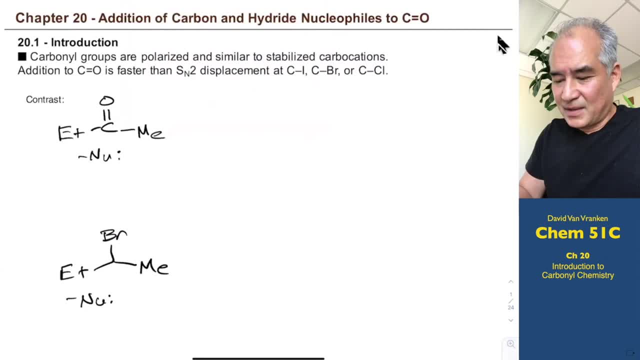 As you know, when you get to secondary alkyl halides, this is not such a great reaction, because you get competing E2 eliminations if you have a strong nucleophile, And then you end up in this sucky situation where you're trying to worry about. 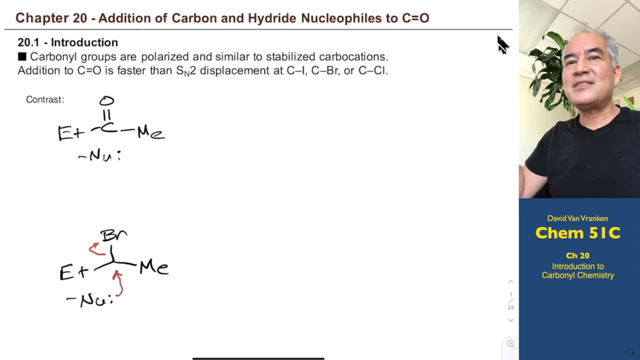 gee, is it E2 or SN2 or SN1 and SN? What a waste of brain cells. that was Because that's not what we don't usually do: SN2 type chemistry, because we don't want to worry about competing eliminations. 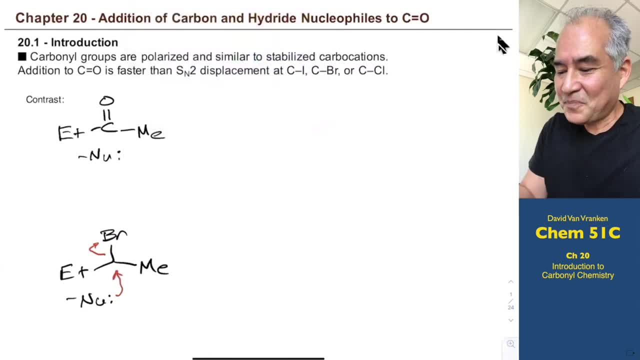 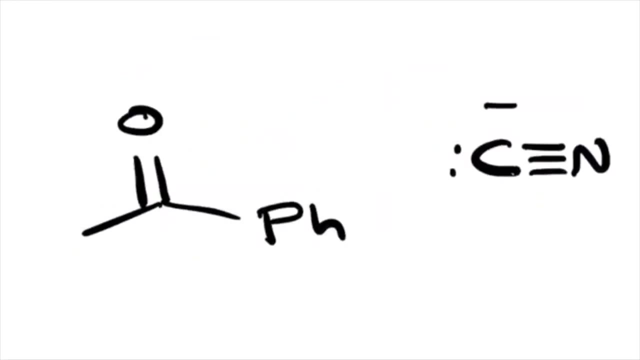 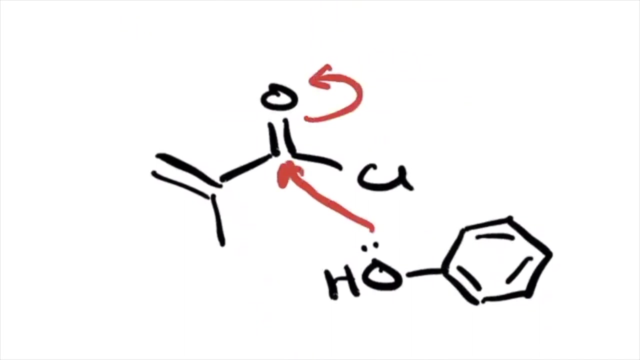 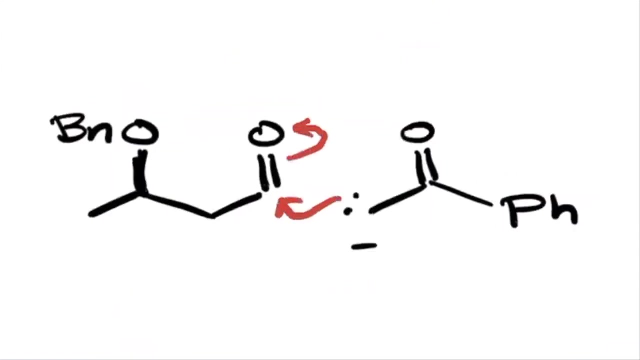 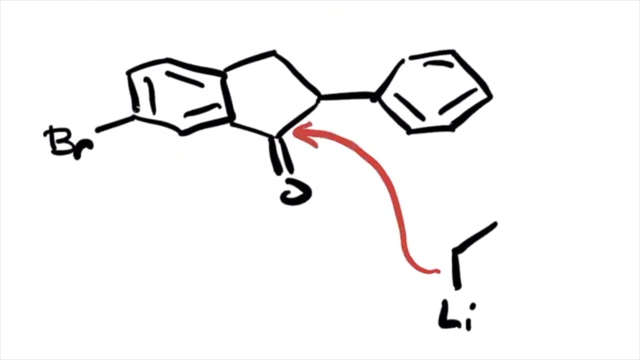 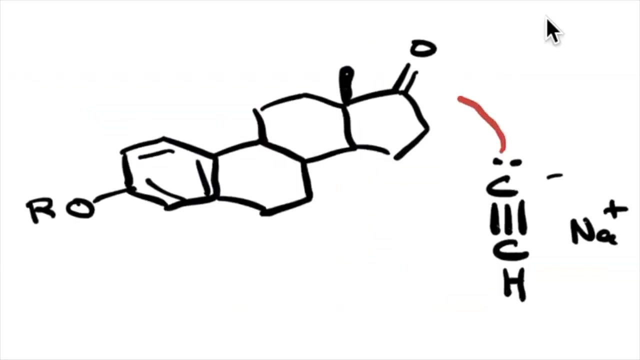 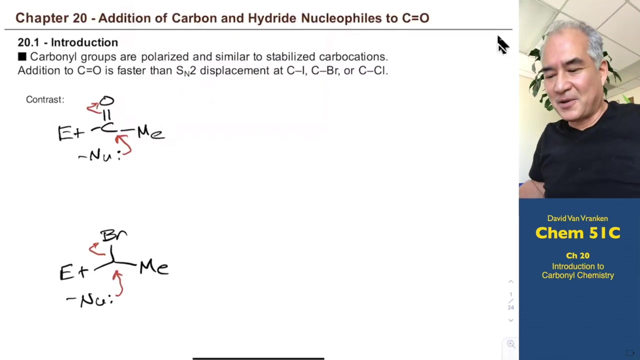 In organic chemistry. what we do is we add to carbonyl groups. Let me come back and change my pen. Here's the way we normally form bonds in organic synthesis. This is the way biology forms bonds. Your biochemical systems work this way. You add to. 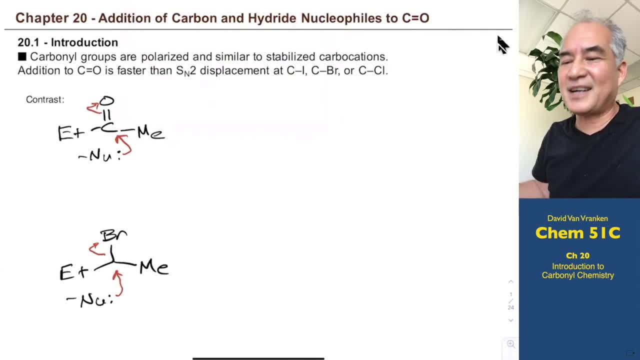 carbonyl groups C double bond O. or if you're making nucleotides, you add to P double bond O. That's the way organic chemistry works. Let's go ahead and talk about these contraindications. Let's go ahead and talk about these contraindications. Let's go ahead and talk about these contraindications. 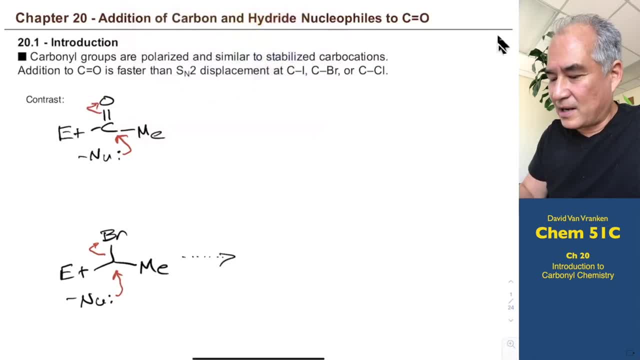 We're going to discuss these two patterns of reactivity. I want to try to encourage you to stop thinking in this fashion where everything you're looking for a leaving group and trying to do SN2 reactions. That's kind of old stuff, That's old thinking and that thinking is not going to. 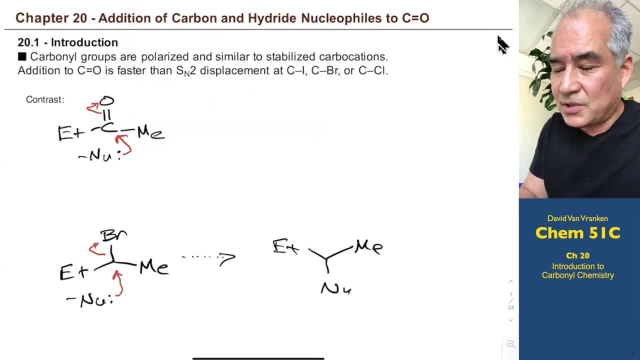 get you anywhere if you're stuck in that mode. What I want you to do first is I want you to think about the resonance structure. for any carbonyl compound, There's a resonance structure that we can draw, where we can take the electrons in the carbonyl group. 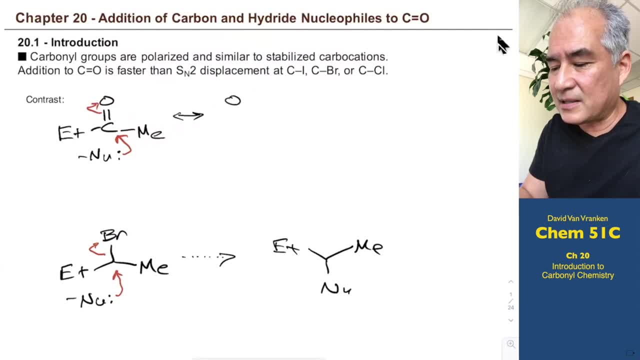 Before I add to that carbonyl, let me just recognize the fact that there's a resonance structure where I bring the electrons up to the oxygen and I draw the CO double bond instead as O minus and C plus. When I draw it like this, I feel like it's a lot more obvious that carbonyl compounds are a lot like. 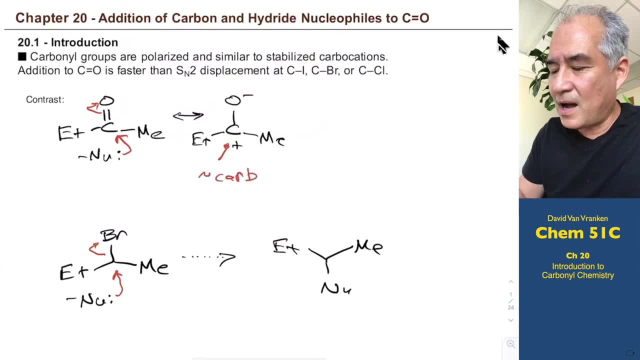 carbocations. I'll just look right here. Wow, that's a lot like a carbocation. You should already know that nucleophiles want to add the carbocations so that carbocation can satisfy the octet rule. If every time you see a carbonyl, you think of it as a carbocation because of this resonance. 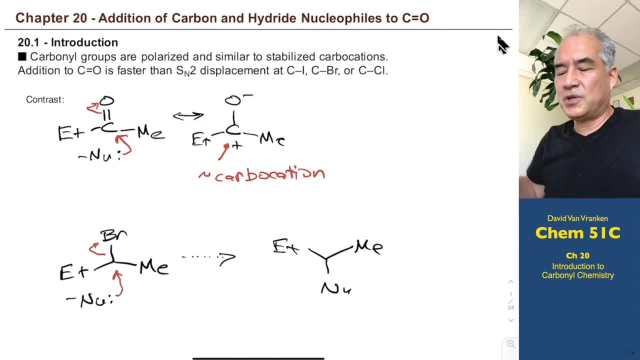 structure, it'll be easier for you to intuit that you should be attacking that carbonyl group. That's what the rest of this quarter is going to be about. is this idea that we're going to add to, instead of doing SN2 every chance we get, we're going to do a process called addition. 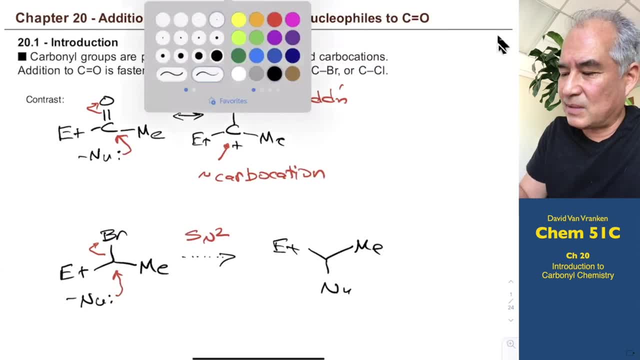 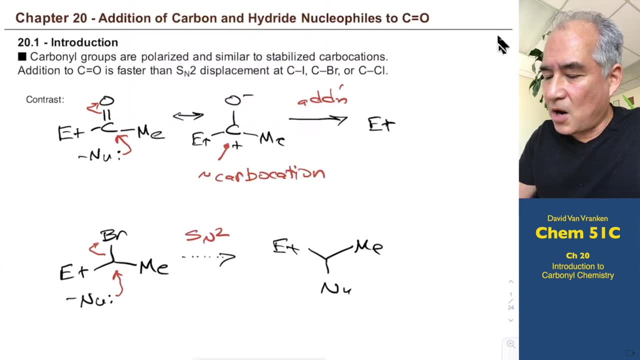 I'll just write addition here With a little abbreviation symbol there. So we're going to add to carbonyl groups and there won't be a leaving group that detaches. but we are going to break a bond in these cases and so we'll end up pushing the electrons up to the carbonyl oxygen. 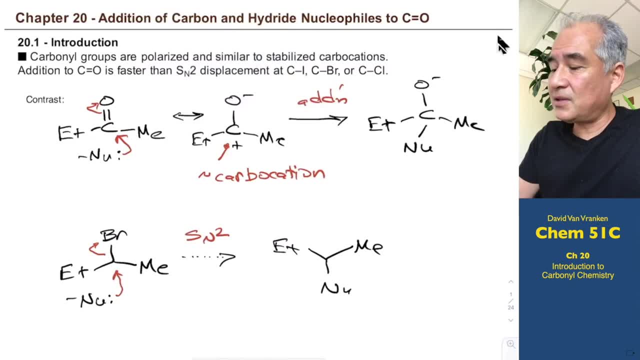 and we'll make a new nucleophile carbon bond. So this is the theme that we're going to be focusing on in chapter 20,, 21,, 22,, 23,, 24, and 25.. Chapter 25 is on amines, but we'll still be adding 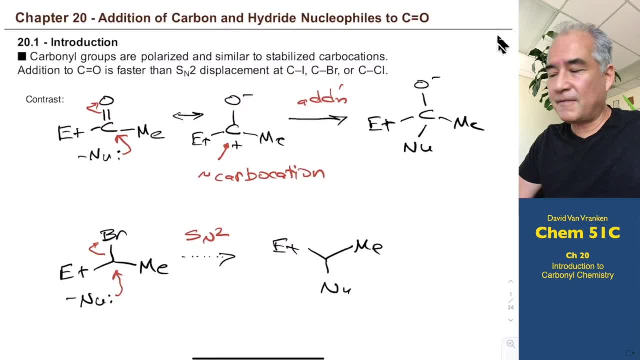 to carbonyls in that chapter. So this is such a difficult transition to make. If it took you nine months just to learn SN2 chemistry and SN1 chemistry, boy, you know we are going to have no time. So let's just wow. add to carbonyls. 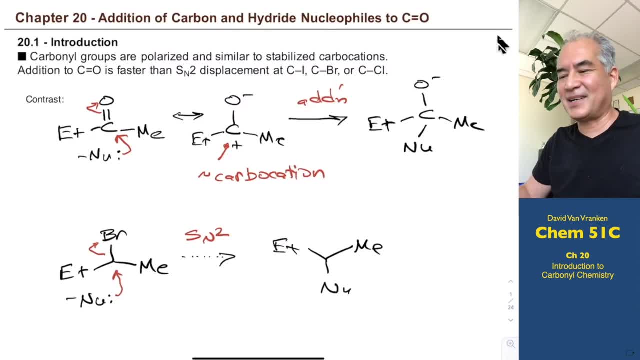 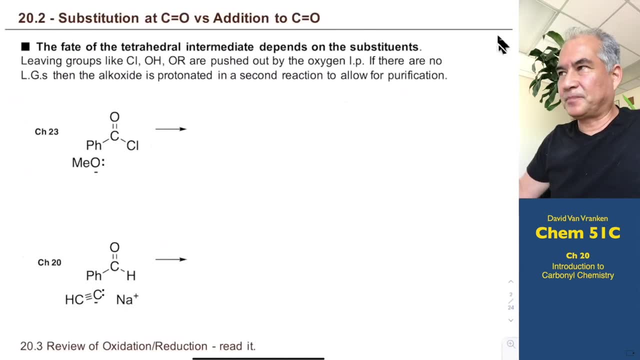 Add to carbonyl groups to make bonds Just cannot emphasize the importance of that enough. Okay, let's go ahead and take a closer look at a distinction between two classes of bonds of carbonyl compounds. So there's going to be some classes of carbonyl compounds. 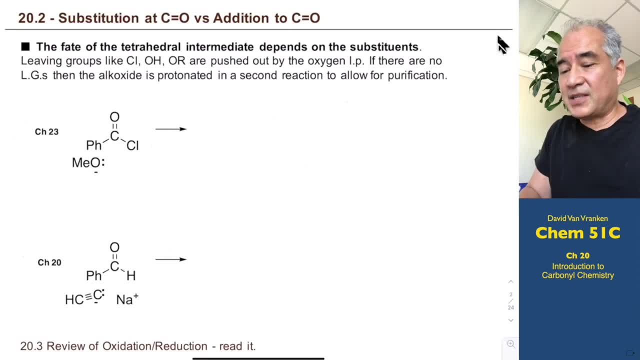 where we have electronegative atoms attached. For example, we might have a chlorine here or an oxygen atom here, OH or OR or in some cases even an amidal. those aren't as good. And then in other cases we'll have an H or an alkyl group. 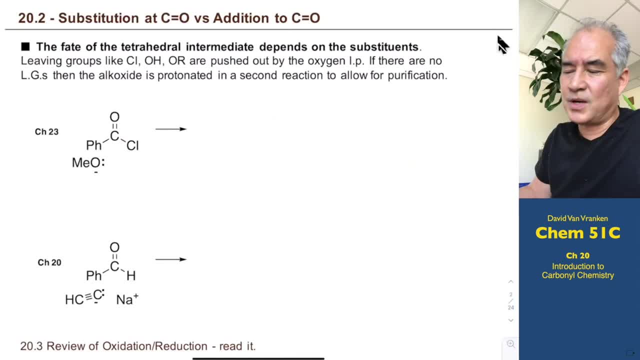 which can never act as leaving groups. in any reactions we teach you in organic chemistry, A simple H or alkyl groups never act as leaving groups. So, depending on whether we have chlorine bromine, iodine or some oxygen substituent there versus H or alkyl, 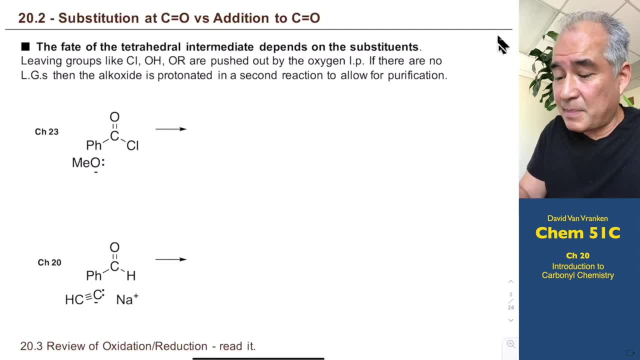 if we have something that's a potential leaving group and it might not even be recognizable to you that that is a leaving group, and we'll teach you how to recognize those things. If there's a leaving group here, the overall reaction that we're going to see. 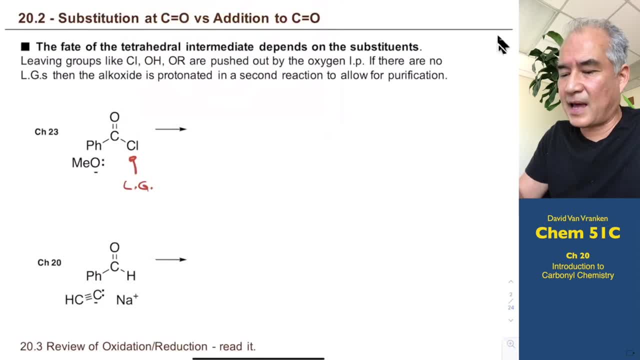 is a reaction of substitution, And I'll walk you through the mechanism for that. So let's go ahead and take a closer look at what would happen here If we have a potential leaving group. here, the first step is always the same, That's addition to the carbonyl. 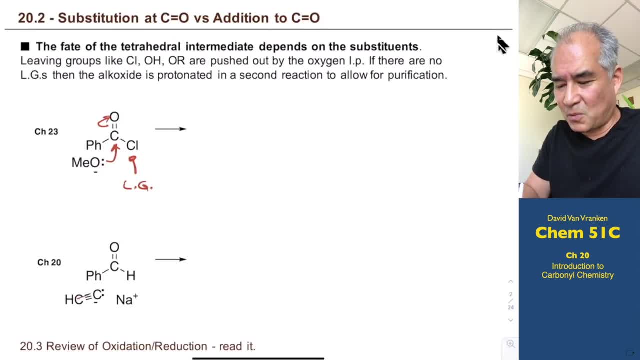 If we take some other nucleo. oh, look at this nucleophile that we learned way back in the alkyne chapter, chapter 11 in our textbook. Remember these acetylide anions and they tried to tell you that you could do SN2 reactions. 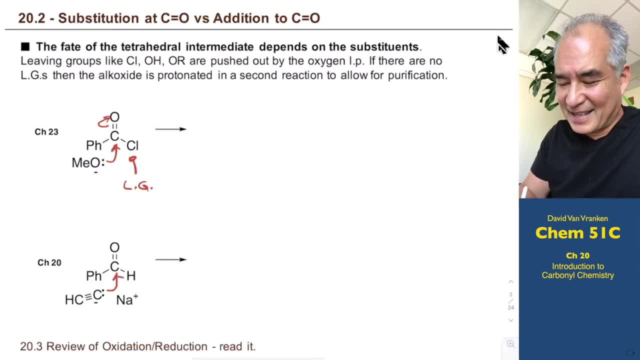 Nobody uses them for that. When people make acetylide anions in the laboratory, they use them to add to carbonyl groups. That's what we use them for in organic chemistry. That's all the first birth control pills. chemicals were synthesized. 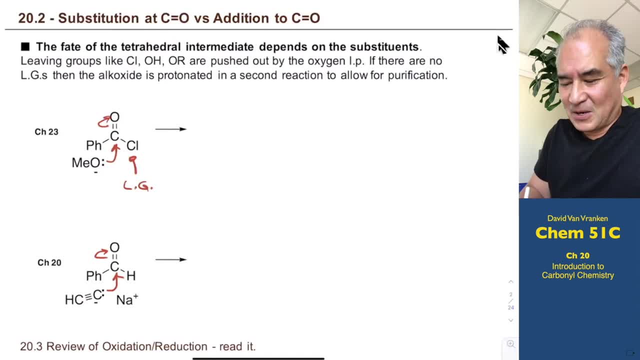 We still use those in the synthesis of pharmaceuticals. So don't forget your friend, the acetylide anion back from chapter 11 in the Gorzinski-Smith textbook. So you want to add to carbonyls, but let me go ahead and draw the intermediates that you get. 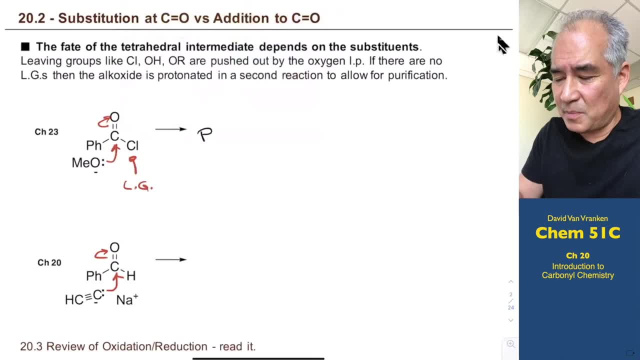 when we add in these two situations, one situation where there's a leaving group and the other situation where there's no leaving group. So if I add them a methoxide anion to this carbonyl, Let me go ahead and draw that methoxy group attached here. 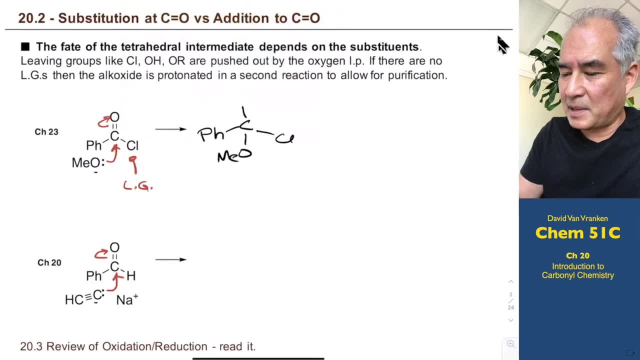 There's the chloride. I'm going to use that as a leaving group in a minute- just not yet. And then I have this oxide anion there. I'm going to draw one lone pair here because I know I'm going to need that lone pair. 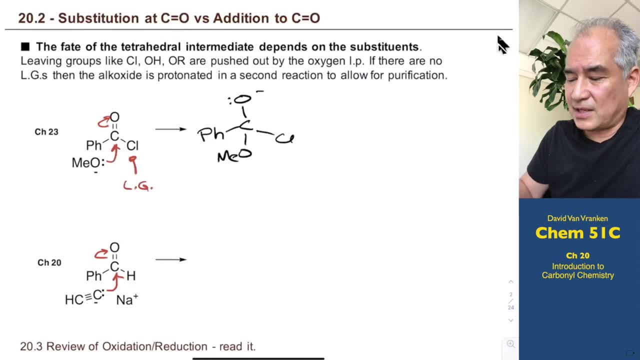 in just a second. We work to refer to this process as addition. So whenever you add to a carbonyl group and you don't have a leaving group leave, you kick the electrons up to the carbonyl group group and we refer to that, that mechanistic step, as addition, and you would do the same thing over. 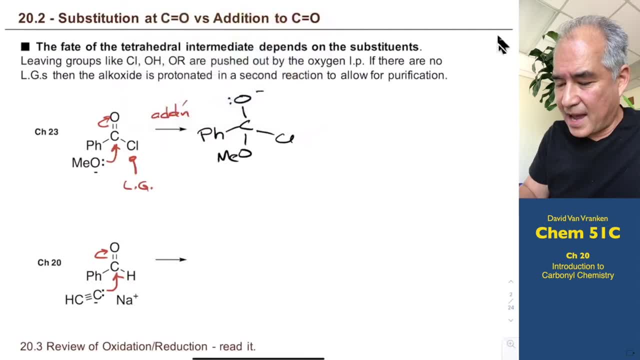 here with the uh, uh down below, when you add to just an aldehyde or a ketone, where there's no leaving group on there. oh my gosh. look at this carbon carbon bond. oh that's just, that is so good. oh my gosh, that feels great to make a carbon carbon bond boy. we've waited. we waited seven. 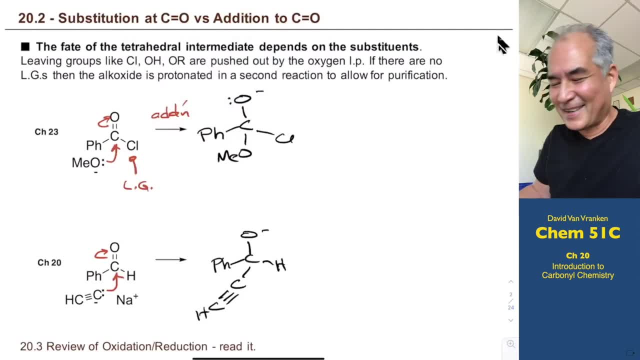 months in the organic chemistry series to make carbon, carbon bonds like that, and finally that feels so good. okay, when there's a leaving group and at an acyl halide, acyl chloride or an ester, or in some cases even an amide, we're going to push out this leaving group here, and so let me go ahead. 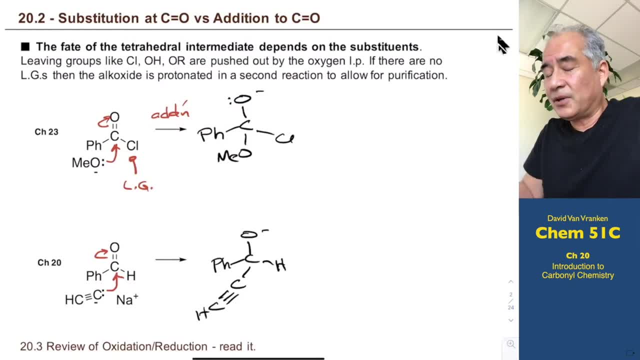 and use that o minus. look, i've got a nucleophile. you kind of learned that you can do sn2 reactions on alkyl chlorides, but if you have an o minus or even a c minus- and we'll show you instances like that later next door- 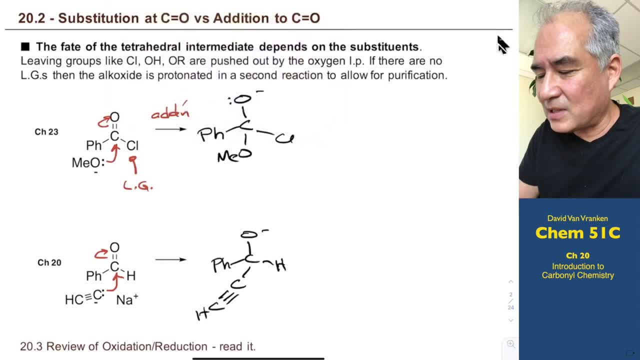 it can easily push out this leaving group. so i just can't wait to use this lone pair. that is right here. it's overlapping in space with the antibonding orbital. it's pushing, it's pushing, it's pushing. the o minus is always there. it doesn't have to collide through an intermolecular. 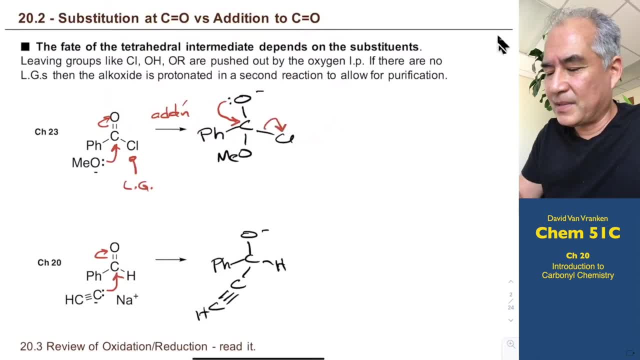 process and it can just so easily push out that chloride. so wow, that's um, that's amazing really what we're. so this is what we're going to see happening with esters and acid chlorides, and we refer to this process as an elimination step. let me write it in red, just so at the 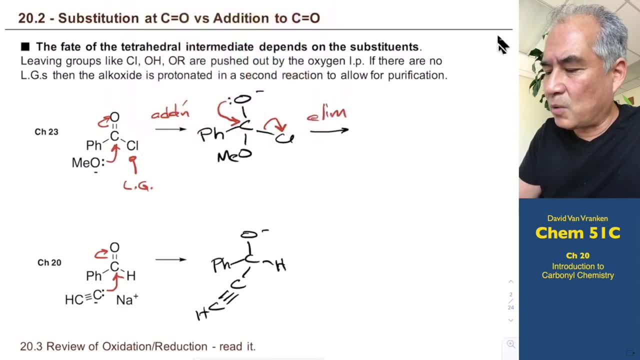 for the sake of consistency i'm not going to write the whole word, i'll just write a linen: elimination there. so this two-step process of addition and elimination results in substitution of the leaving group. it's not a one-step process, it is not a one-step sn2, but you can substitute. 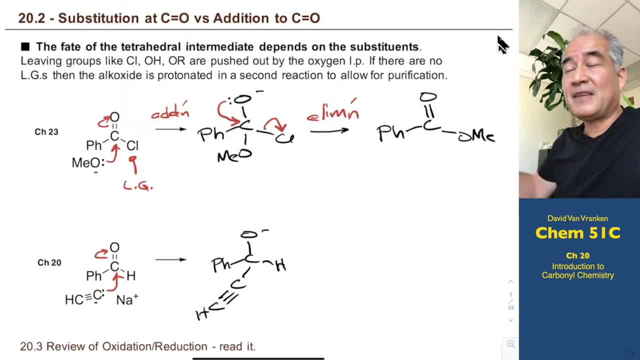 leaving groups on carbonyls like chlorides and leaving groups that you're, you're. that aren't going to be comfortable to you yet, but notice how we've, in a, in a two-step mechanism, we've achieved substitution of a substituent that was attached to a carbonyl- big time theme coming up. 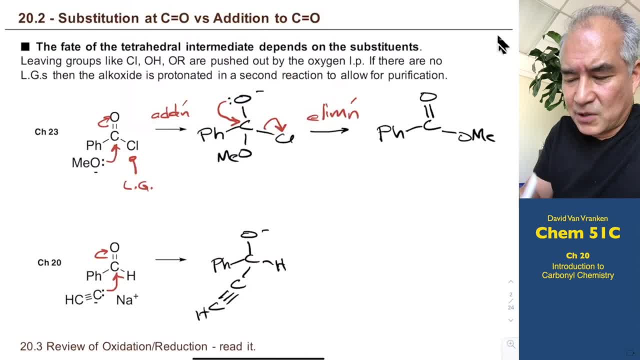 uh, in chapter. uh, i think that's going to be chapters 22. um, let me change this. i think that's chapter 22 in the fifth edition of the gorzinski smith textbook. okay, when there's no leading group on there, right, we, we, we have lone pairs over here on the um, on this oxygen down below, when we add to: 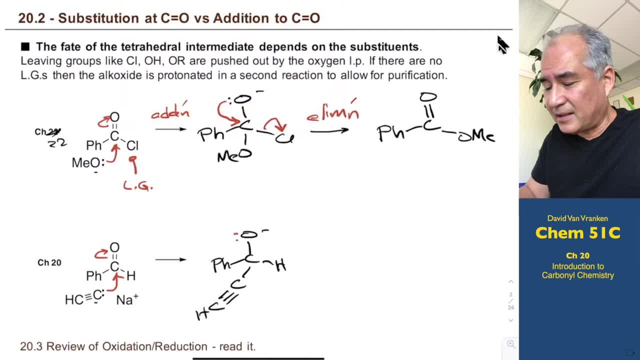 an aldehyde or a ketone, but they can't push out any leaving group. there's nothing here that's recognizable as a leaving group, so we're going to push out any leaving group, and we're going to push out any leaving group, so that'll just sit there, and sit there, and sit there you'd still. 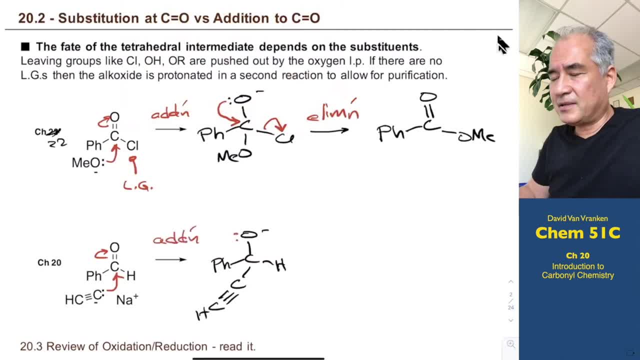 refer to this first step as addition, but this is just going to sit there until we work up the reaction. there's a, a sodium ion, in there that's just floating around waiting to. nothing's going to happen with that, so that'll just sit there and you can come back a day later and dump some water. 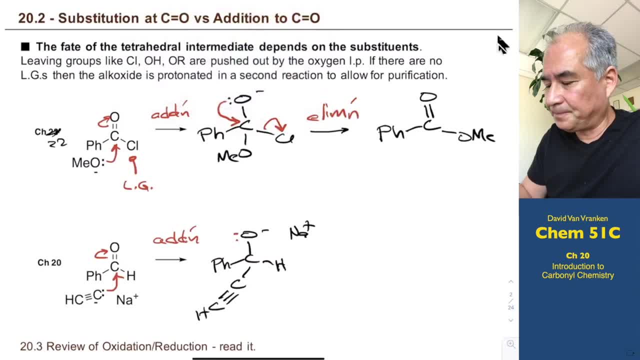 in there and what will happen is, when you dump some water in there, i'll write h2o and i'm going to write the word work up. we're not adding the water to try to do sn2 reactions or anything fancy. we're just dumping some water in there, swamping it with. 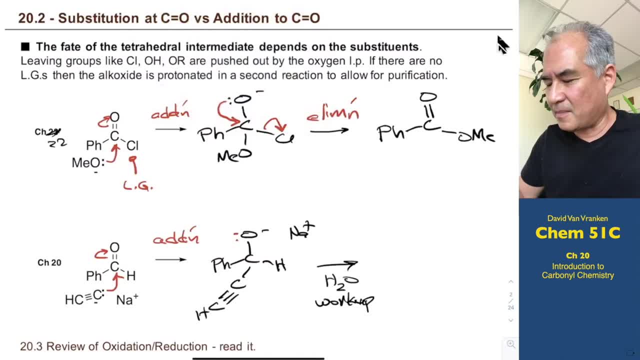 water to try to protonate it. you just take a beaker full of water or dump some water in there and you can protonate that o minus and then you get a neutral molecule. and this is really the goal for organic chemistry is to get neutral products that we can extract into organic solvents so that 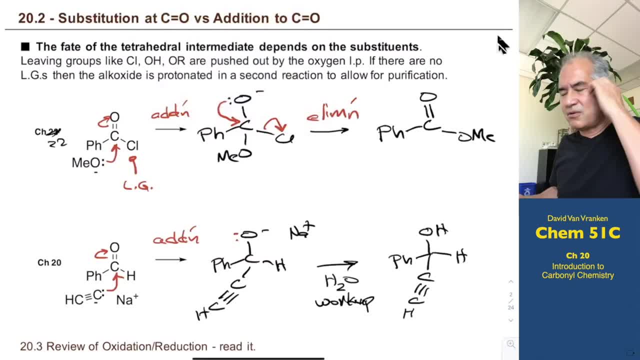 we can evaporate the organic solvents. i'm not going to draw the stereocenter, of course that's. that's formed as a racemic mixture, but we'll talk about that a little later. so there's two steps here. in when you do reactions of ketones and aldehydes. but it doesn't substitute the h or 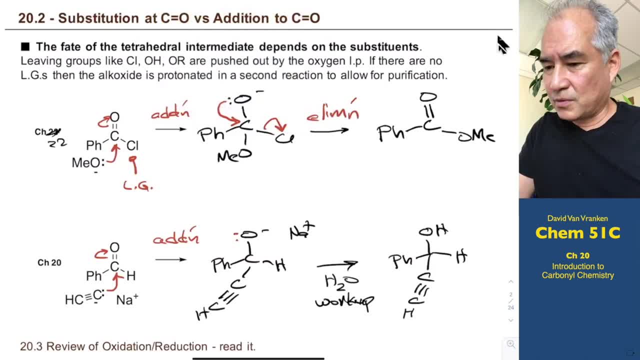 the phenyl on the original carbonyl. so just just note here that this is a two-step process. it's step one is add, and then you have to remember to come to include the fact that you're doing an h2o workup when you add to an aldehyde or a ketone. okay, let's go ahead and take a look a. 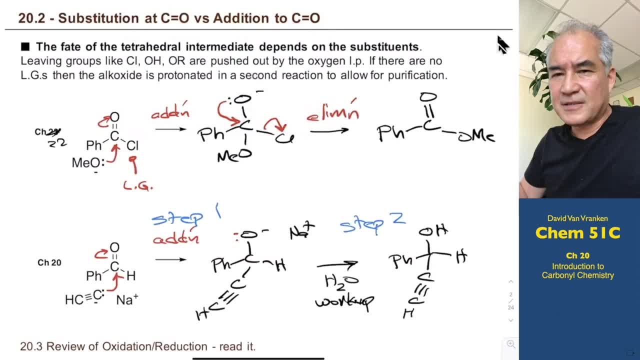 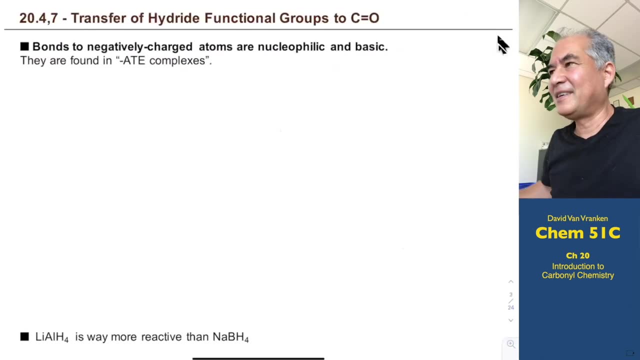 little bit further here at a, at a class, the first class of nucleophiles that we're going to show you. so what's new about this chapter? we're teaching you to add to carbonyl groups. add nucleophiles to carbonyl groups. that's what organic chemistry is all about. that's what it is all about. i cannot say that enough. 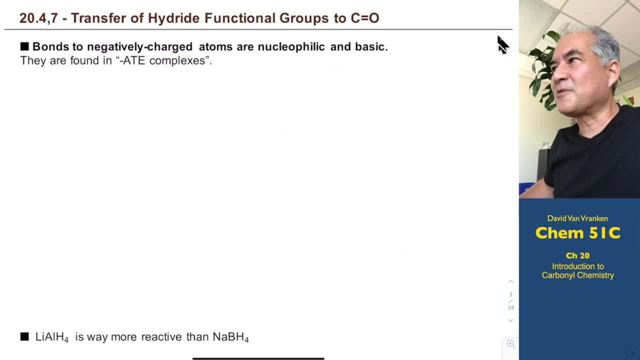 okay, let's take a look at the first weird functional group. that, um, that i don't think you have seen before. you might have seen hydrido borates if we, if you covered oxy mercuration reactions. i can't tell you how many of you have seen that. i can't tell you how many of you have. 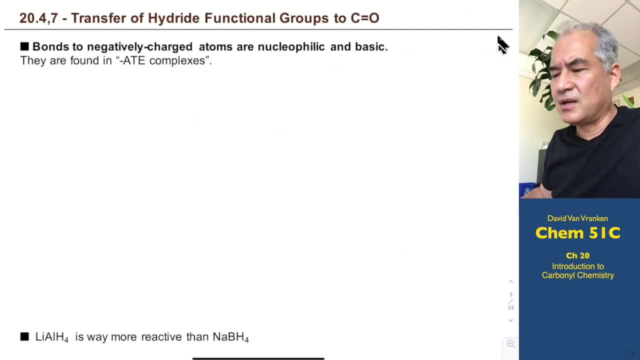 seen that i can't remember whether that was covered in the addition to alkene section, uh, but you didn't use it as a nucleophile. and here we're going to teach you how to use eight hydrido eight complexes as nucleophiles. let me go ahead and show you those two hydrido eight complexes that 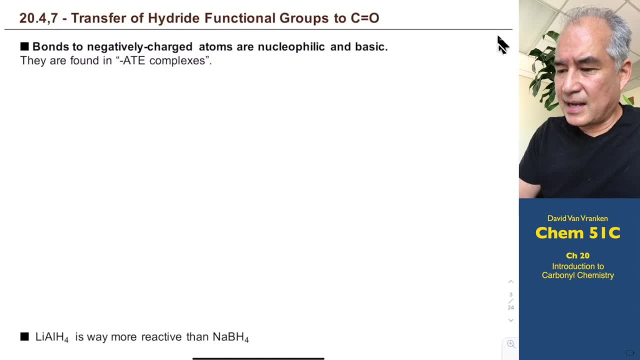 you're going to learn about one of one of these reagents and i have to just think up for a moment here about how i'm going to depict this. um has has these long- i'm going to draw this freakishly long- these long nucleophilic bonds to aluminum. now, aluminum normally only wants three bonds, but you know. 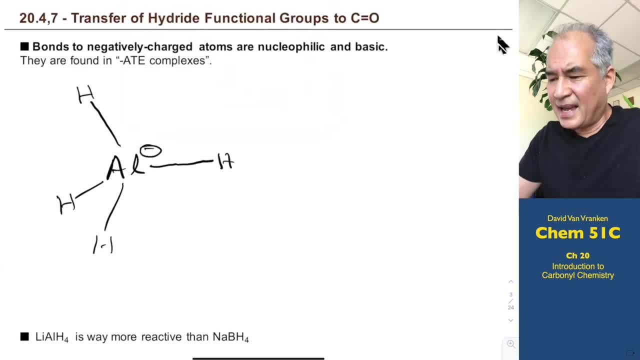 they sell this reagent where it's got four bonds, so it's got a negative charge, and they sell this as the, as the lithium complex, the, the sodium tetrahydrido aluminate, doesn't have good solubility, so it's not as common. uh, so lithium, this is called lithium tetrahydrido aluminate. 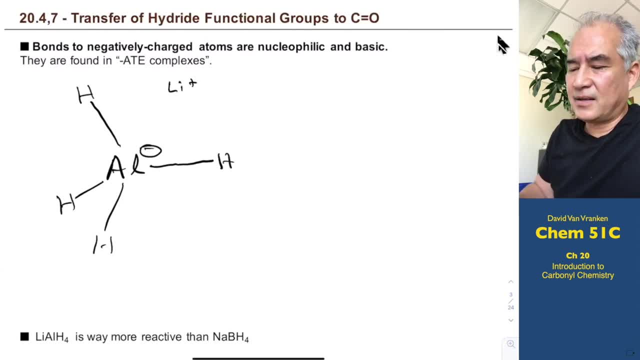 would be the formal way to describe that, and the word illuminate eight tells you there's a negative charge in the aluminum um they also. another common reagent is sodium borohydride and i'm going to draw these bonds normal sized. these are like typical second row atom type bonds. 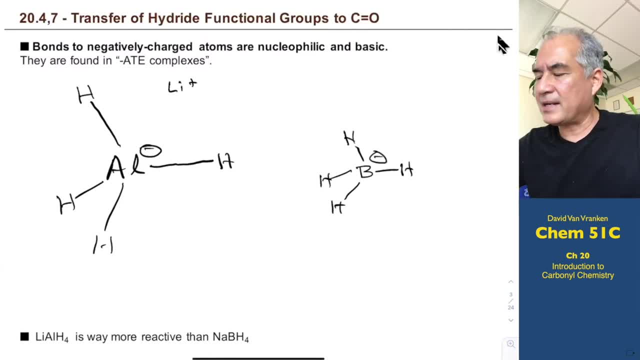 boron's in the second row. this is tetrahydrido borate, also called sodium borohydride, but i like the word hydrido borate because i like to focus on the fact that there's a negative charge. borate tells me there's a negative charge. 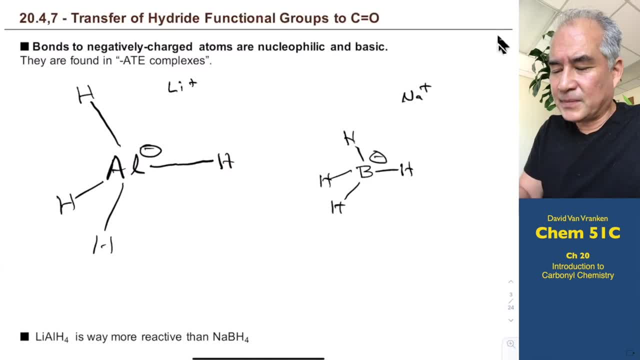 on boron. look, when there's a negative charge to aluminum on aluminum, that means all the bonds to aluminum are nucleophilic. so, and it's not the aluminum that is going to form bonds, it's going to be the h's that form bonds, that h is going to want to attach to other things, that h is going to. 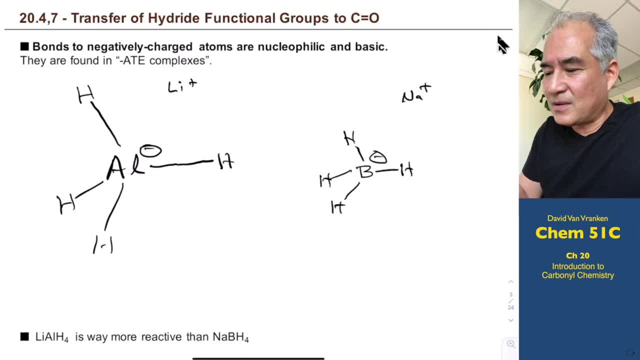 want to attack carbonyl groups. now, these two compounds are not equally reactive. the one with the longer bonds, and this is generally true in organic chemistry: when you have longer bonds you are more reactive, and if you have way longer ponds, then that means that this, this tetrahydrido illuminate, is way way more reactive. 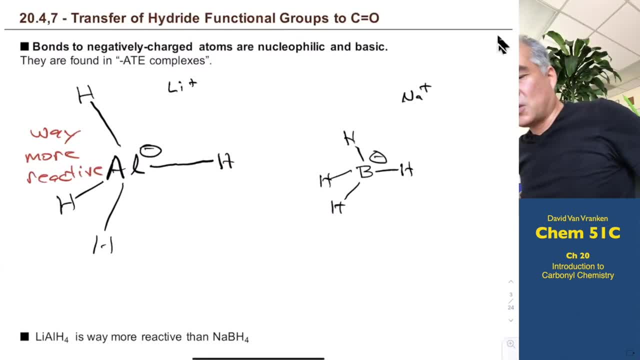 than that tetrahydridoborate, so way more reactive. and these bonds, these h atoms, these hydrido groups, the h's, are going to want to attack things. so let me go ahead and just draw this out here, that we're you know, we're trying to focus on these bonds here. those bonds are nucleophilic, the bonds. 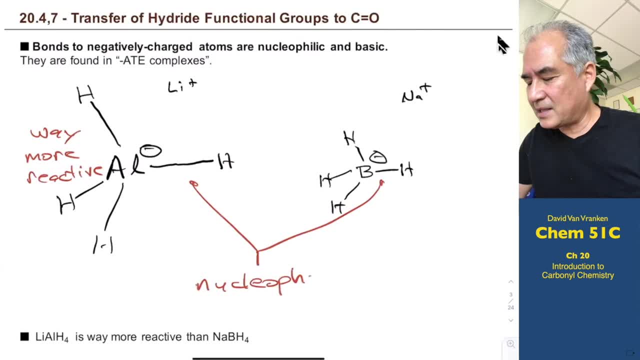 themselves are nucleophilic and it's going to attack other things like the hydrogen and the hydrogen and it's the h's that are going to be attacking things. okay, so here's two reagents that you haven't seen used before as nucleophiles, and these are going to be total money for you. i, i. 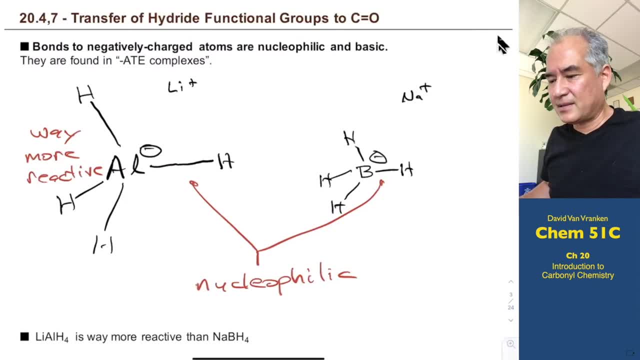 promise you i'm going to have some version of this on my final exam. i don't know what problem i'll make up. if you go to any exam in any organic chemistry course, the final exam at the end of the year is going to have these reagents somewhere there in the exam. you just have to know how to use. 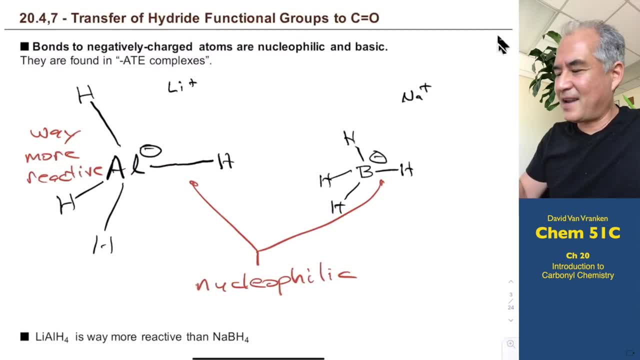 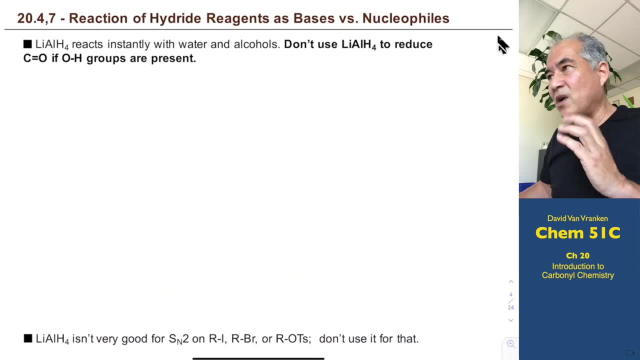 these in every single circumstance. you just have to know how to use these in every single circumstance, and there's lots of ways to use these reagents. so let's get started. i'm using tetrahydrido boric reagents, so i'm going to start off by what you don't want to do. let me start off with the more. 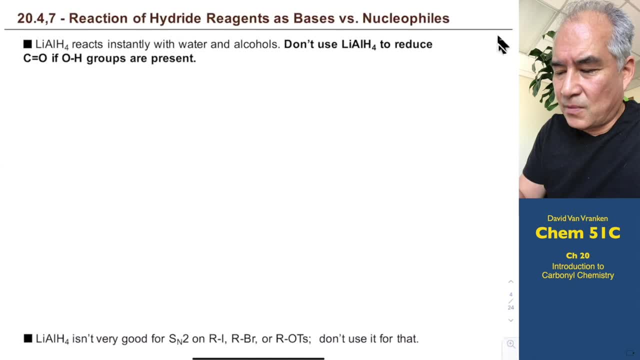 reactive one, which is tetrahydrido aluminate. so i'll start over here, kind of in the middle of the page, where i draw this tetrahydrido aluminate reagent. i'm not going to draw the bonds freakishly long here just to save space. but this is that tetrahydrido aluminate reagent, and here's one. 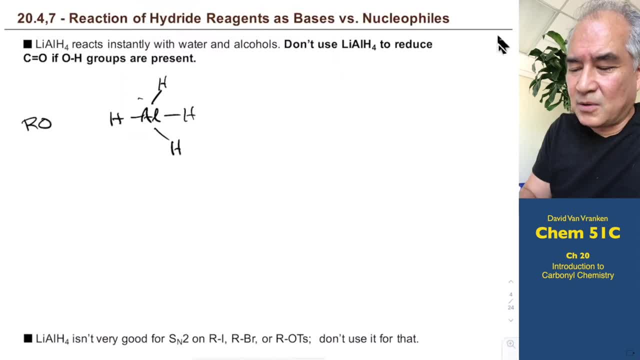 thing you would never do. you would never put this reagent in water or in an alcohol, because you're just going to destroy the reagent. because what will happen if you do that is, these long nucleophilic bonds are also long and basic, and so they will instantaneously deprotonate the water or the alcohol, and they will do it so fast. 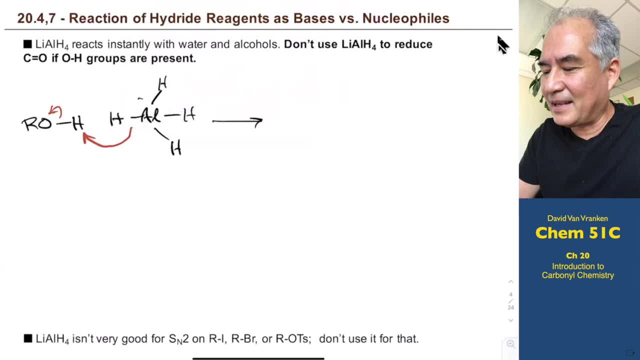 and so aggressively and so exothermically that, as you generate hydrogen gas, notice it's the h that's forming the bond here as you generate hydrogen gas. this thing is going to be so fast that it's going to be so fast that it's going to be so fast. 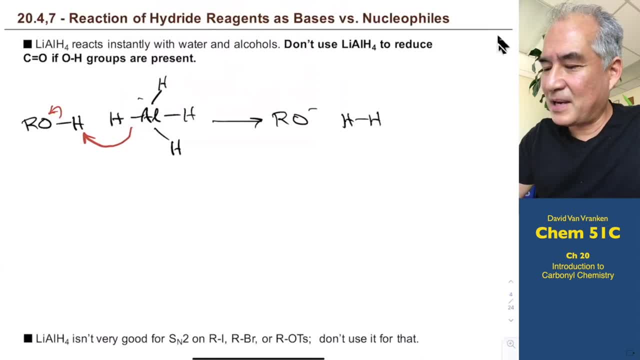 this thing is going to burst into flames, so i don't know how to. how do i draw? can i draw a flame here? i don't know if i can draw flames. flames, the hydrogen gas from the heat would catch on fire and and catch. then if you had anything else flammable in there, you would end up with a fire. so we would. 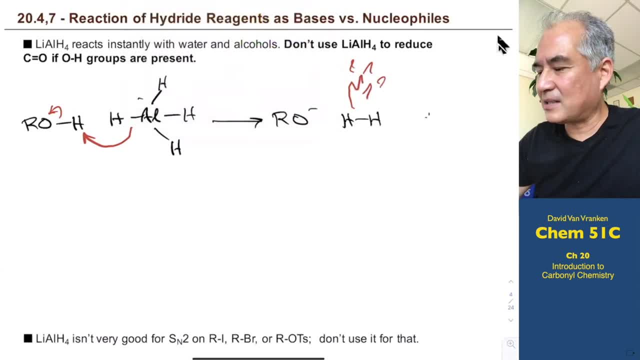 never expose a super aggressive reagent like tetrahydrido aluminate to to to either alcohols or to water, because it would destroy our tetrahydrido aluminate reagent. um, and that's not what we use, tetrahydrido. 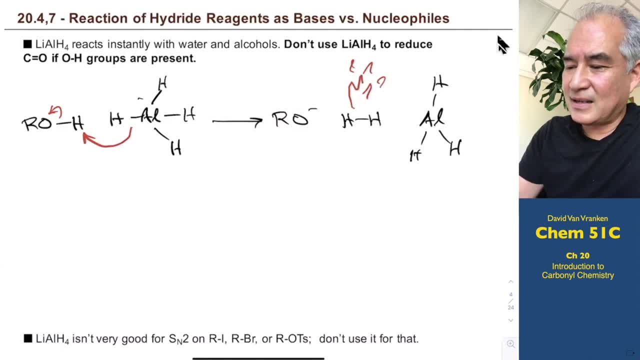 illuminates for the. the idea here is that if you have a tetrahydrido, illuminate and if you exclude, keep it away from, if you exclude things like water or oh groups, as long as you can exclude those and you have a carbonyl within a thousand miles. 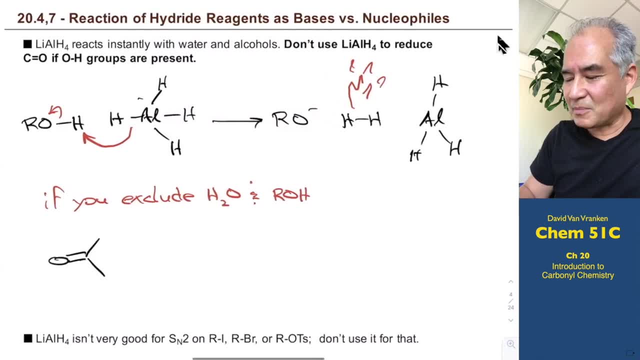 you're going to add to the carbonyl group. that's what we do with carbonyl groups. this is what tetrahydrido illuminate reagents are super useful for. this is what you're going to be using them for for this quarter. is you're going to be taking those tetra? sometimes i circle my 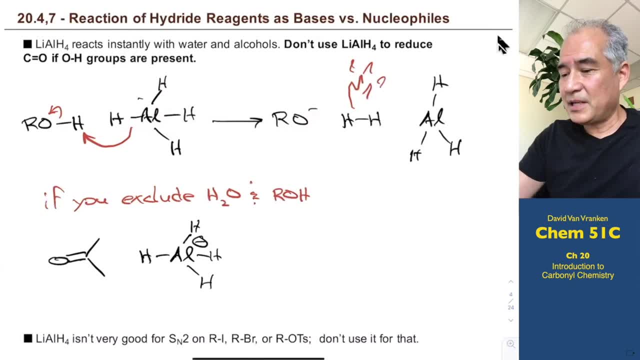 charges if i'm worried you won't see them. um, we're going to be using these tetrahydrido illuminate reagents to form bonds between the hydrogen and the carbonyl carbon. remember, carbonyl carbons want to be attacked by stuff. that is what we're doing this quarter, and so you'll end up forming. 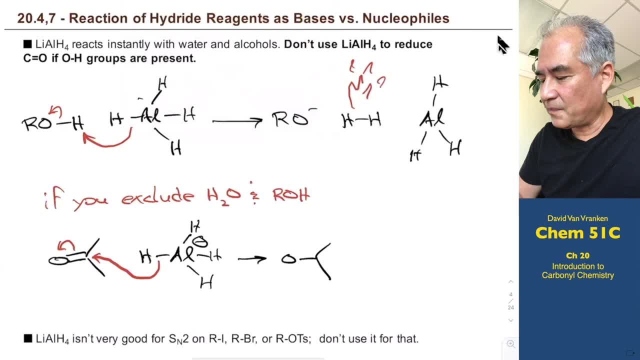 if you start with a key ketone, you'll end up forming an alcohol. Initially you'll form an alkoxide, but this is the idea, And it's easy to protonate an alkoxide. dump a bunch of water in there and you'll. 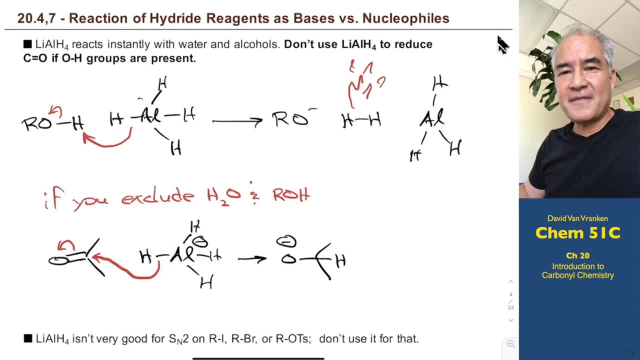 protonate it. So it's kind of the opposite of an oxidation. You learned how to use PCC and chromic acid to oxidize alcohols to carbonyls, and now we're showing you how to go back in the other direction. And again there is a byproduct here. This species is called allane. It's kind of like. 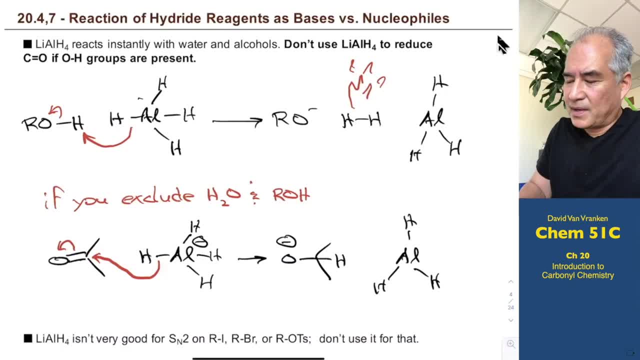 methane, but aluminum only wants three bonds. So this tetrahedral aluminate is a super powerful and aggressive nucleophile. but that's not to say that you should be using it for SN2.. It is not very good for SN2.. Don't try to use lithium, aluminum hydride, lithium, tetrahedral aluminate. 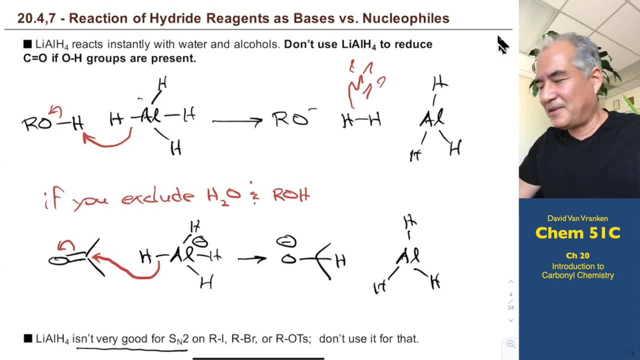 for SN2 reactions. If you're doing that you're thinking you know you're kind of it's not useful for those reactions They you have to use. to get that to work you'd have to use some special conditions solvent systems. 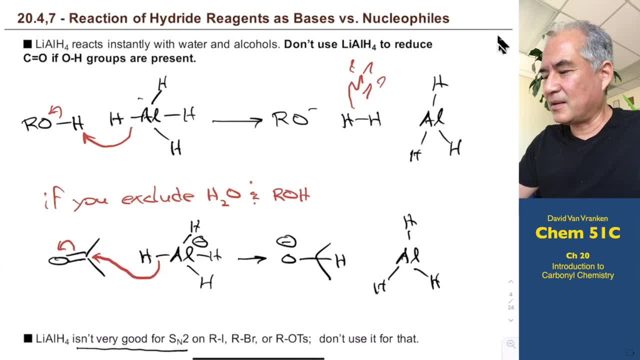 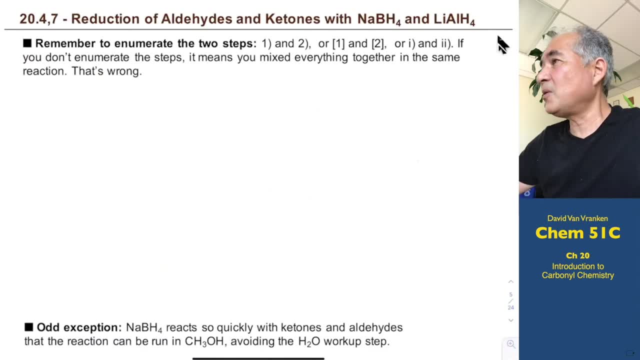 that we don't talk about in this quarter, So those tetrahedral aluminates for reducing carbonyl groups. Now let's go ahead and think a little bit more about how we're going to use these reagents, And I am going to have to teach you about enumeration of steps, And I don't think 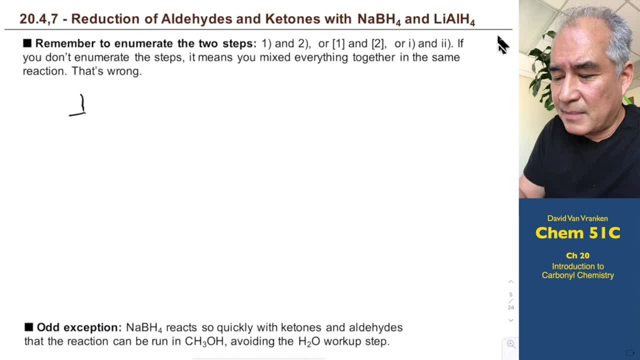 we've made a big deal about that yet. So let me go ahead and take a substrate, and I'm just going to pick one that looks kind of weird to you. Why? Just to try to get you to think outside the box. Okay, what do I see here? Yeah, there's a cyclobutane ring. Forget that, there's a carbonyl. 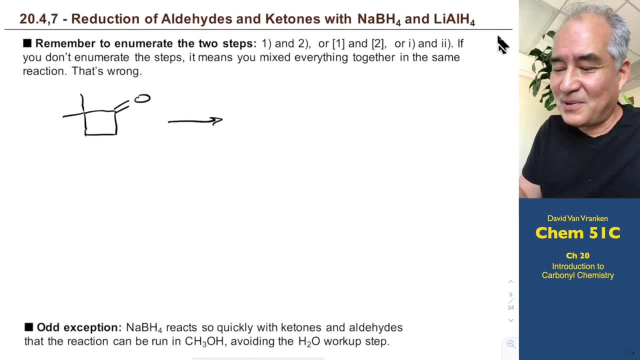 Don't you want to add to that carbonyl? I sure do, But as soon as I see that carbonyl, I want to add a nucleophile right in there and make a bond. Okay, so if we wanted to convert this to an alcohol? 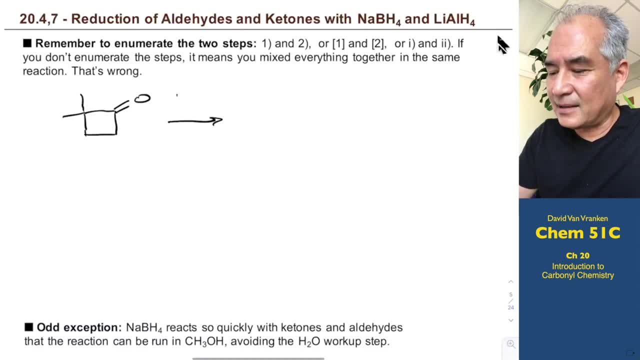 then we use lithium aluminum hydride. Just go like this: It's easy: Lithium aluminum hydride. But that will give us an alkoxide anion And you know we're going to have to figure out how we're going to do this. 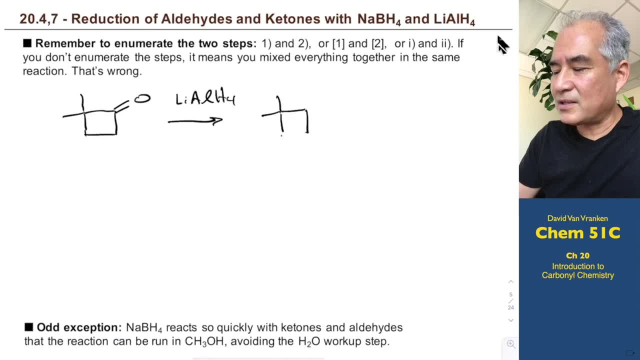 And organic chemists don't want to work with insoluble salts like lithium alkoxides. What we want is neutral alcohols that we can extract into organic solvents and then evaporate the solvents and we've got pure compound. So we have to follow this up, as I just indicated. 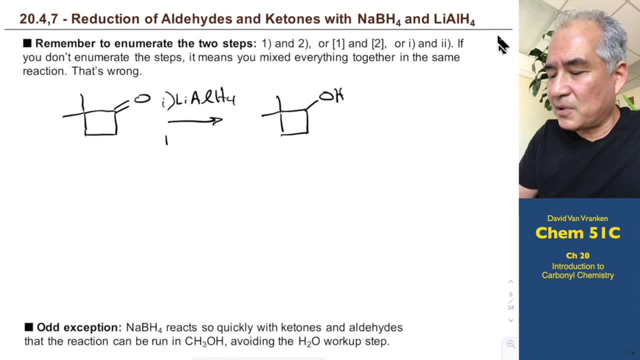 in that previous slide is we have to follow this up with an aqueous workup. If we want to put a proton on that O minus product, then we have to write that in here, And the book will often do it like this. I like to write the word work up there. 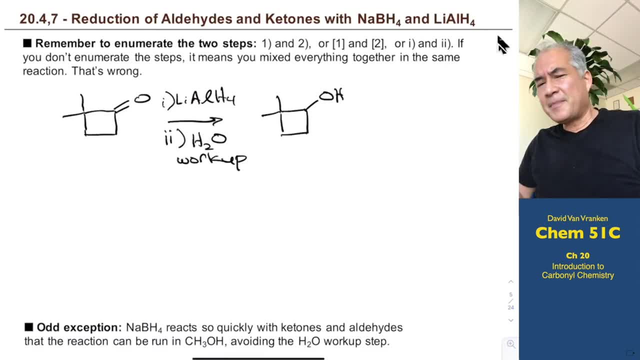 to make it absolutely clear. It's like: what am I doing with that water? I'm not trying to do SN2 or SN1 or use it as a nucleophile. I'm just swamping it with water to stick a proton on the O minus because nobody wants to isolate salts. You have to enumerate the steps, Step one: 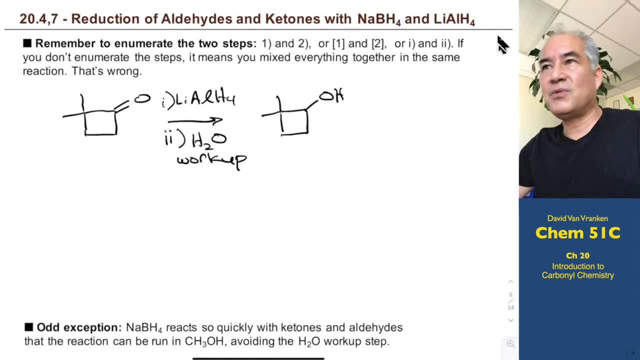 you add lithium, aluminum hydride, You go away for lunch. You come back after lunch as your reaction cools, whoarks back up from being in an ice bath, the flask being in an ice bath. then you come and dump your water into the reaction. So these are two independent steps And let me 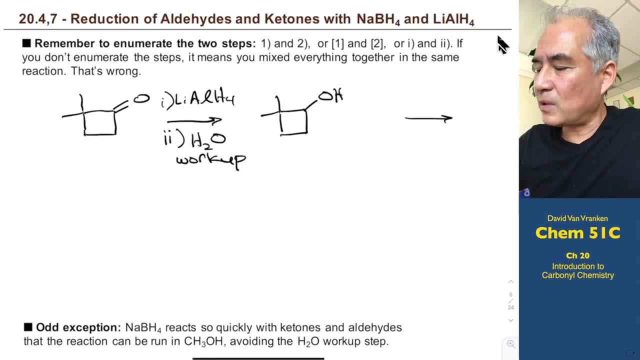 just make it absolutely clear here that if you write this out without enumerating the steps one, two, if you write it out like this and you don't put numerals of some kind there, then that's completely wrong. That is absolutely and completely wrong. I already told you what. 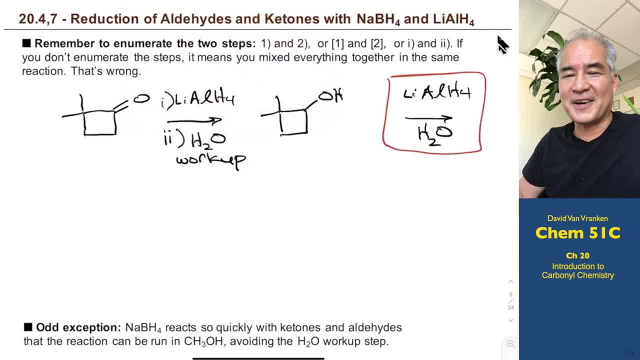 happens if you mix lithium aluminum hydride with water. I'm sorry, That's not the way I'm gonna write this in. I'll see you soon. Thanks for watching. if you mix lithium aluminum hydride with water, the hydrogen gas catches on fire. 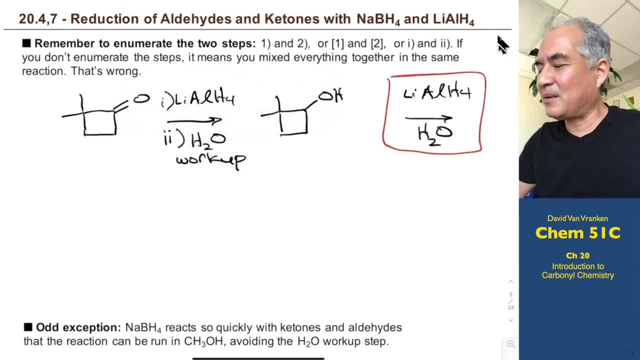 and you wouldn't get any of the carbonyl reduction. you would simply destroy your lithium, aluminum hydride reagents. So this is totally wrong to write this out, so I'll just write totally Wrong. that's wrong. You have to enumerate the reagents. 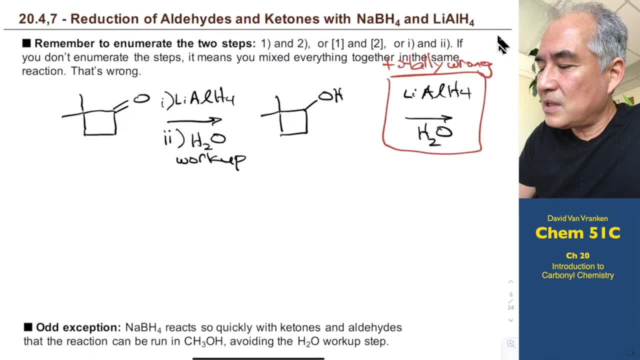 Now the book enumerates the reagents using these brackets one and two, And you'll find that I sometimes enumerate my reagents using Arabic numerals one and two with little parentheses. there I usually use small Roman numerals to indicate I'm not trying to isolate the products in between. 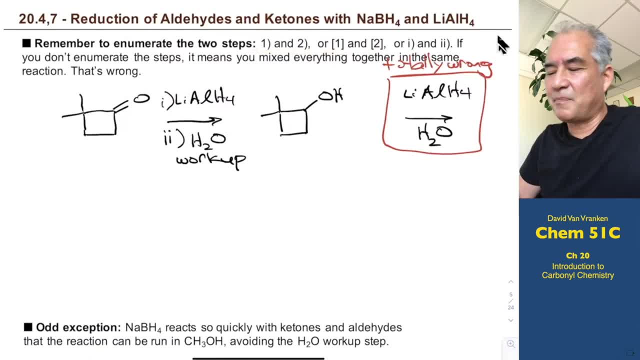 and purify them. It's just like when the reaction's done, you dump in the steps in Roman numeral two. But if you used any of these types of enumeration systems, that's fine, Just to make it absolutely clear to anybody else that you're not dumping everything in there. 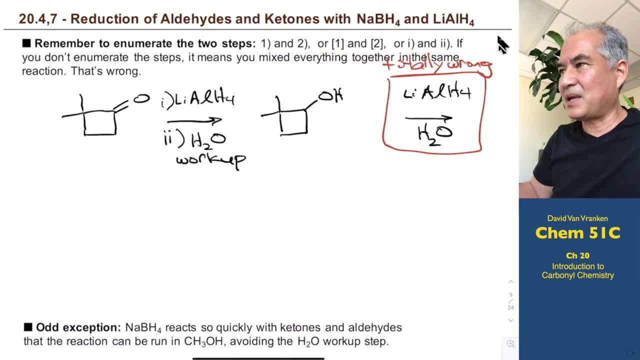 at the same time. If you don't enumerate it, then it indicates you're dumping everything in there at the same time. Now I'm going to encourage you to do the same thing with sodium borohydride, just because it's easier to remember. 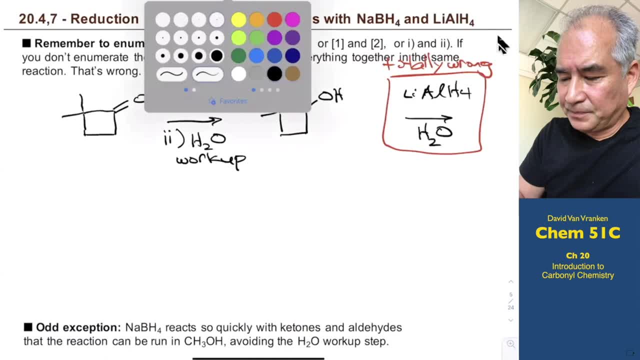 So let's go ahead and draw out with this idea here that, if you have, you can do the same thing- reduce ketones and aldehydes. And so let me just kind of highlight this here: You can reduce ketones and aldehydes. 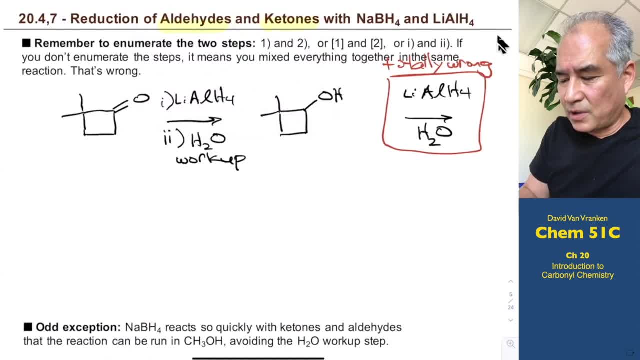 aldehydes and ketones with sodium borohydride or lithium aluminum hydride. So if we take, I'll do an aldehyde this time, just to be different. So if we take an aldehyde and we treat that, we can do another two-step process with sodium borohydride. 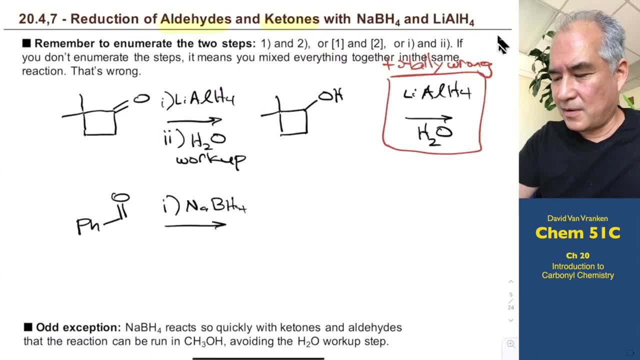 and follow that up with an aqueous workup. That's the worst looking four. Let me see if I can correct that. There we go. I think that looks like a four, And then we follow that up with an aqueous workup. 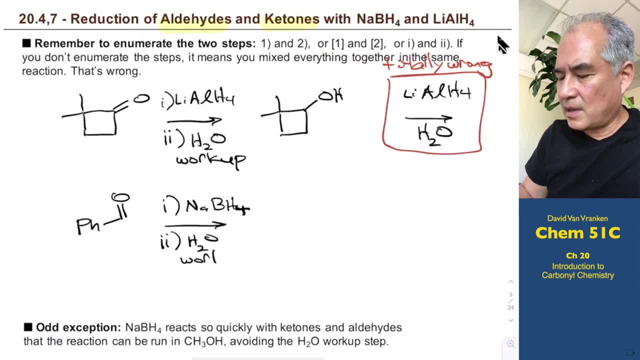 to protonate the O minus that we generate. Again, you don't have to write the word workup, but because, if you're just now learning about these two-step procedures without aqueous workups, I just want to make it clear. 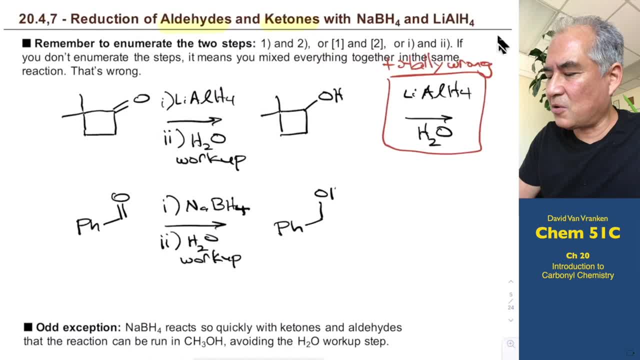 we're not using the water for anything other than just to stick a proton on the O minus so we can get a neutral alcohol product. Now it just so happens that sodium borohydride- and you couldn't possibly have intuited this- 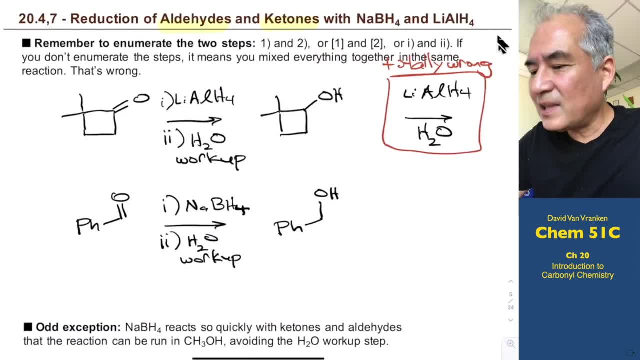 sodium borohydride is so much less reactive than a lithium aluminum hydride. There's a special secret set of conditions that you can use when you use sodium borohydride, and that is this special instance If you're reducing aldehydes and ketones. 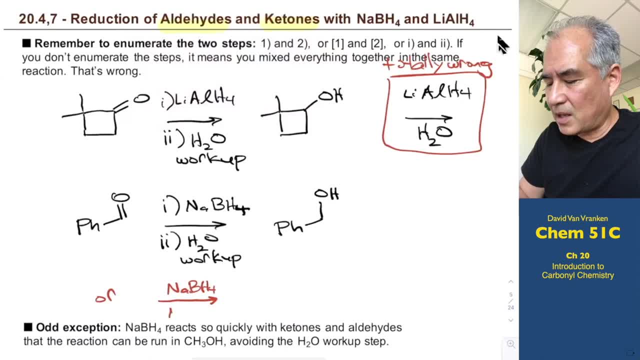 you can use sodium borohydride in methanol. I'll write it M-E-O-H or you could write it C-H-3-O-H, without enumerating the reagents. It turns out that sodium borohydride decomposes. 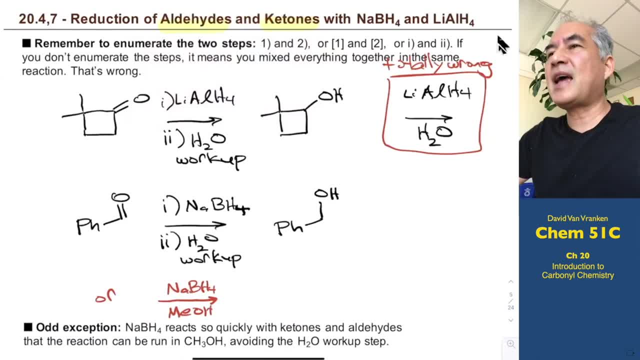 it reacts with the methanol so slowly that you can actually add to carbonyls faster than sodium borohydride deprotonates the methanol. So don't do that with lithium aluminum hydride, Only with sodium borohydride can you do this one step. 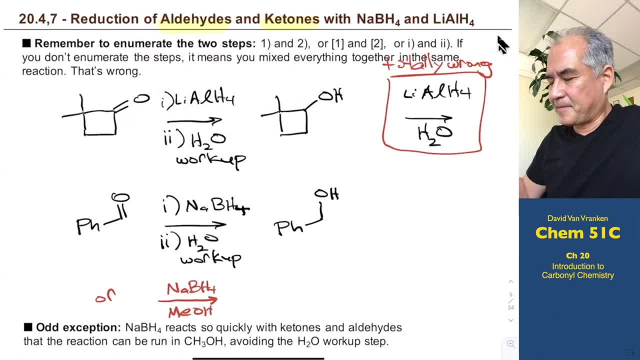 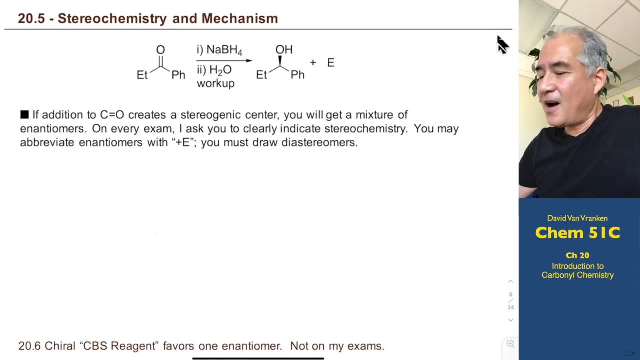 sodium borohydride in methanol procedure. I feel like it's easier for you to memorize if you always do this as two steps, So this would be okay if you did it in that way. All right, we need to talk about the fact. 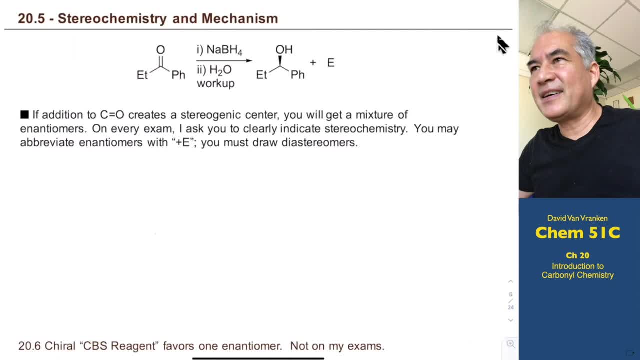 that you end up forming a lot of stereogenic centers when you add to aldehydes or ketones. So let's talk about this When you make a fourth bond you have to think about. did I just put four different substituents? 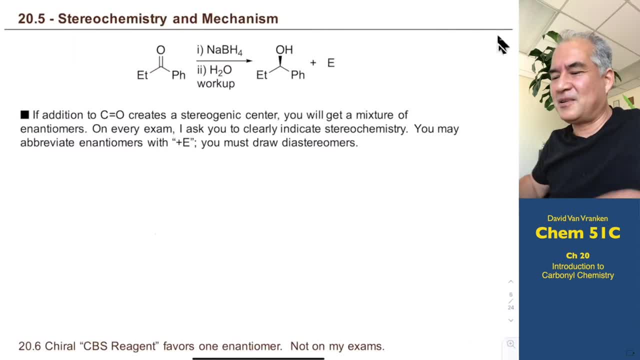 on a carbon atom, on an SP, Because if you did, you've generated a new stereogenic center that wasn't there before. So here's an example of above where, if you do a sodium borohydride reduction of a ketone, 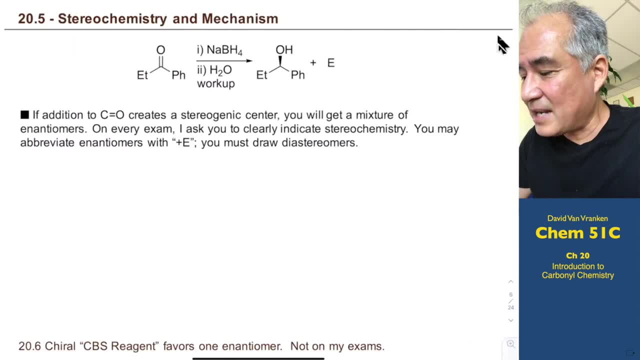 then you'll end up forming a new bond here- And I didn't draw the H, but clearly there's a fourth bond here- And if you have four different substituents on that carbon, then that means you formed a stereogenic center. 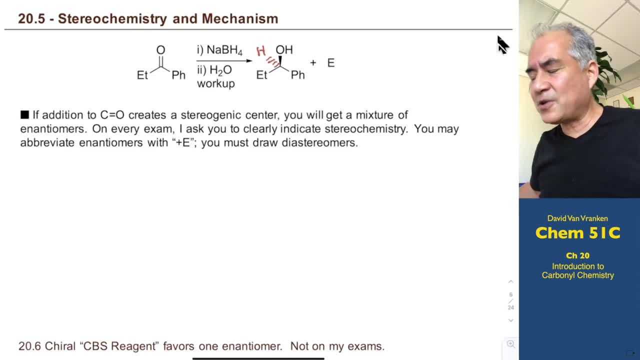 And unless I say otherwise, unless I say: don't worry about stereochemistry, you need to indicate that there's two products to this reaction. There's the alcohol with hydroxy up and then there's the mirror image with hydroxy down. 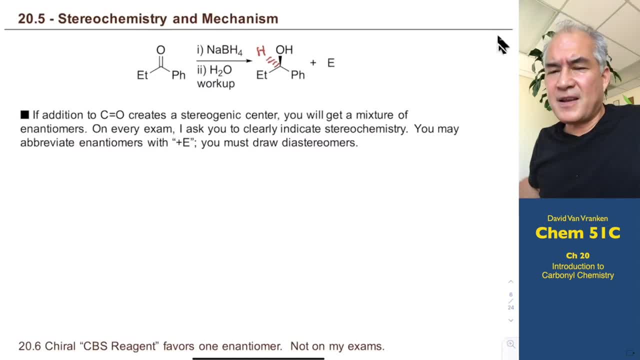 If you're writing this out on paper and you write plus E, every organic chemistry instructor knows that you mean the mirror image and you don't have to draw it. But really the correct- you know the correct- way would be to draw the structure. 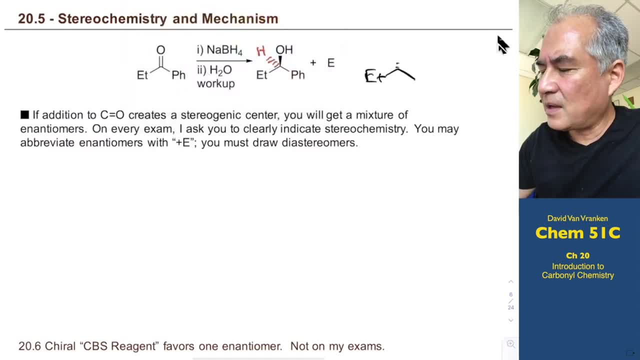 of the of the матon, the mirror image like this, and just draw that. you also, in equal amounts, generate the product where the OH is going down, And in that case the hydrido group added from the top face of that molecule. 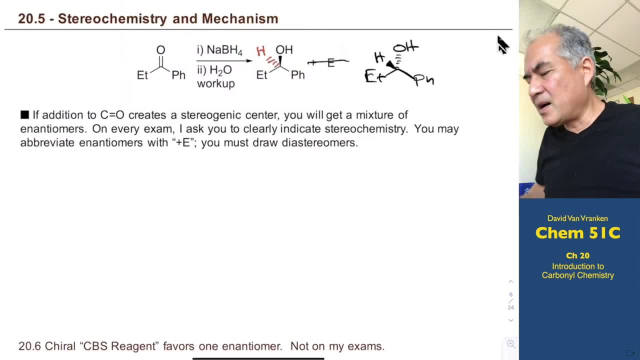 those are mirror images. You would get both of those products in equal amounts. So let's go ahead and talk about this, this, what's going on here? right? If you, if you have, if you have a ketone of any kind, 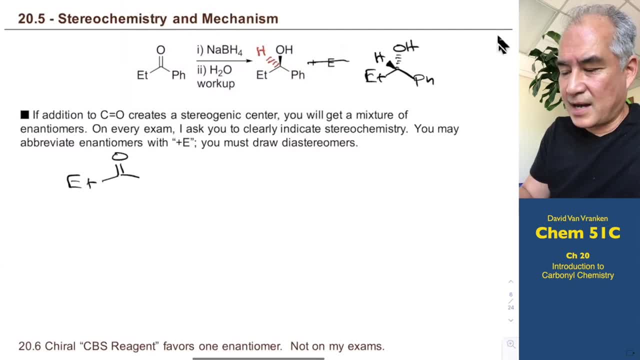 where the substituents are not identical and you add a nucleophile that that makes a third different substituent. I'll go ahead and draw the hydrido borate species like this: And now let's go ahead and add that bond in. 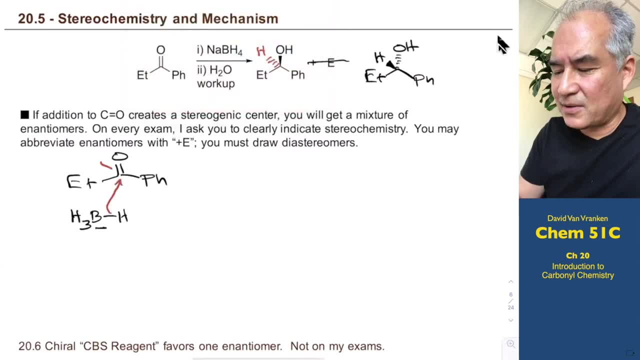 Boy, I just love drawing out this nucleophilic addition to carbonyls Just feels so natural. That's boy. that's what organic chemistry is all about is the addition of nucleophiles to carbonyls. And it's a little bit weird for you because 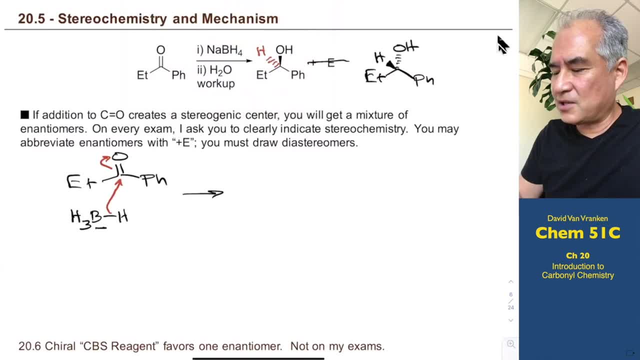 because I know these hydrido borate and hydrido aluminate reagents aren't really what you're used to seeing at this stage. So there's two different faces to this carbonyl. There's the bottom face and the top face. 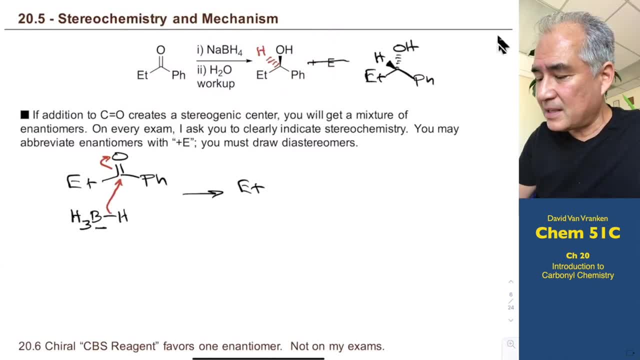 If the hydrido group adds in from the top face, I would need to indicate that. So let me go ahead and draw in that this hydrido group. Oh, I just want to change the way I'm indicating the stereochemistry here, that this: 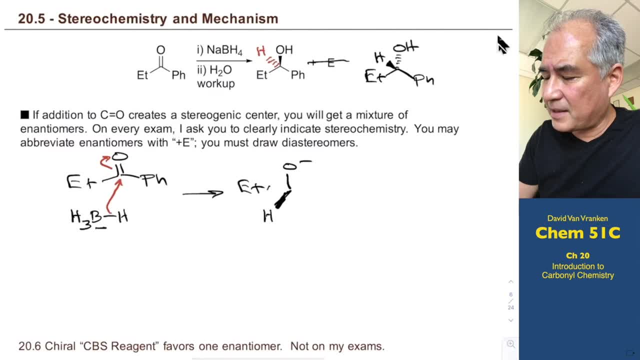 hydrido group added in from the top face And I'll make the ethyl group point backwards. I could have also made the phenyl group point backwards, but that's not what I had in my initial notes. So the so one product would result 50% of the molecules. 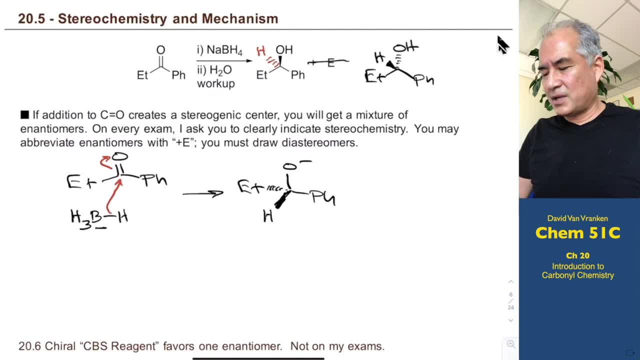 Let's suppose you have 6.02 times 10 to the 23rd molecules in your flask. You know, half of those the hydrido group is going to add from the top face and the other half the hydrido group is going to add from the bottom face. 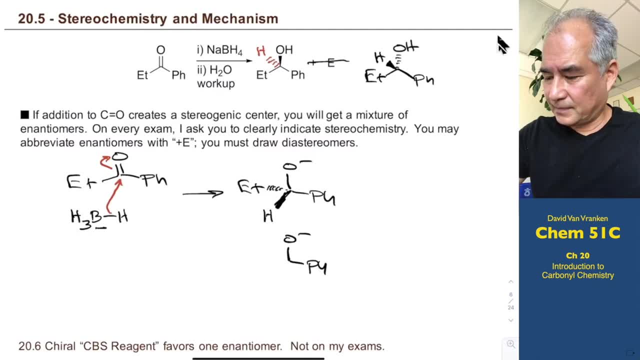 So let me go ahead and draw that, draw that in. I'll be a little more careful writing there. So the other half, that hydrido group, would add in from the bottom face, And now I would draw the ethyl group pointing up. 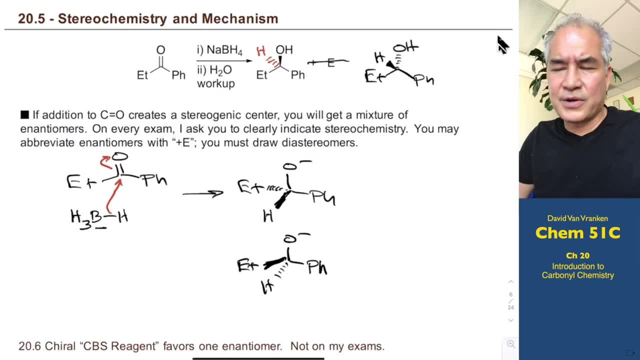 You know there's, there's multiple ways I could have drawn the enantiomers. as long as you're you're you're careful to check the SNR conningle pre-log assignments, You could have drawn these enantiomers in other ways. 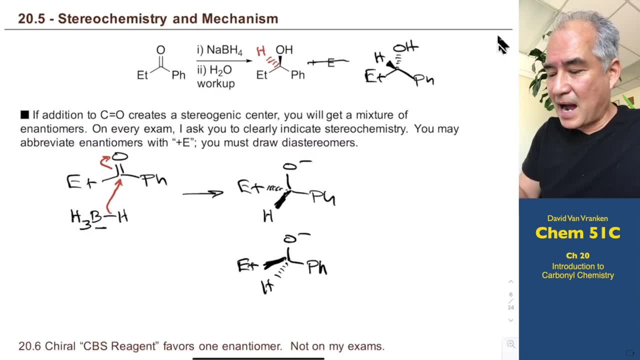 Um, so now you've got a whole flask, right. You usually buy sodium borohydrates- There was a sodium cation in there- until you'll have this whole flask full of sodium salts that you don't want. What you want to do is you want to make neutral molecules that you can extract. 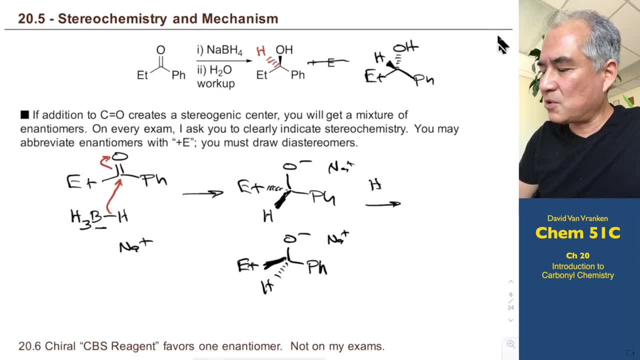 into an organic solvent, And so you just swamp this with water. You dump a bunch of water in there. You know, if there's a thousand times more water molecules than all coxides, then you're just eat by equilibrium. You're going to protonate almost all the own. 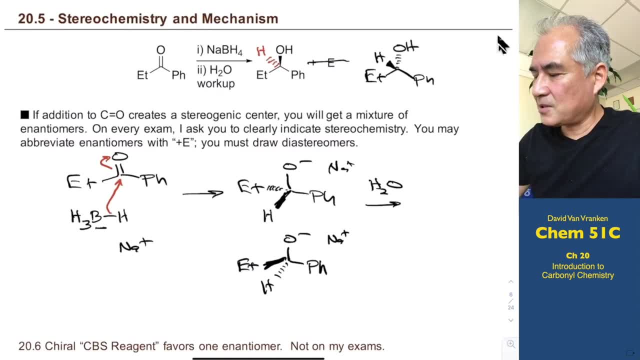 the all coxides, And so this is just a workup here, And so, at the end of the day, what you would end up generating is a mixture of a racemic mixture of two different enantiomers when you generate a new stereogenic center. 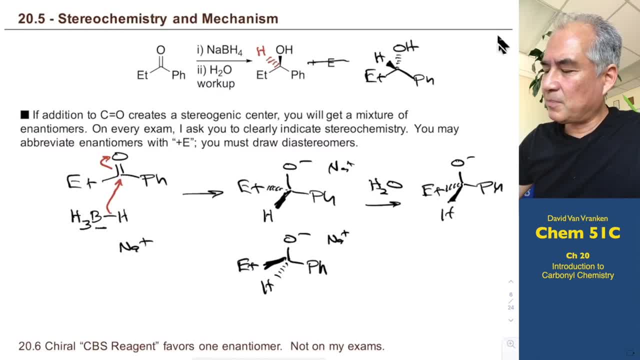 So always look when you add to carbonyls to make a fourth bond, to see if you created a new stereogenic center. I'm just going to write plus E here And I think I meant to make that into an H, So that's a neutral alcohol. 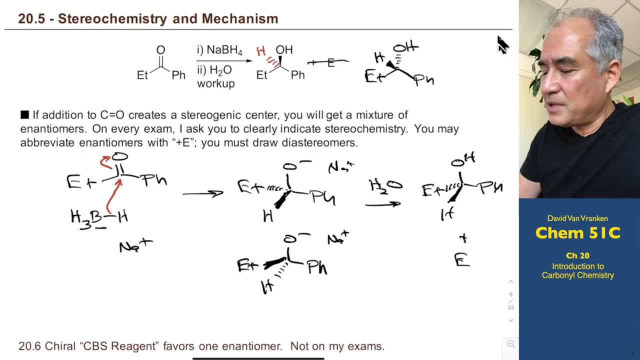 So the product here would be racemic. Now I wrote here that you may abbreviate enantiomers with E, with plus E, but that doesn't work on this sapling online homework system that we're using, So let me go ahead and take that out here. 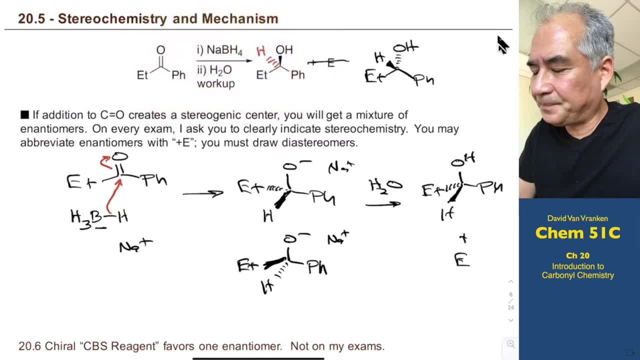 just to be clear that you can't do this. on sapling, You may abbreviate enantiomers with plus E. I'll just write. because this quarter we're taking our exams remotely using this online system. I'll just write. not on sapling. 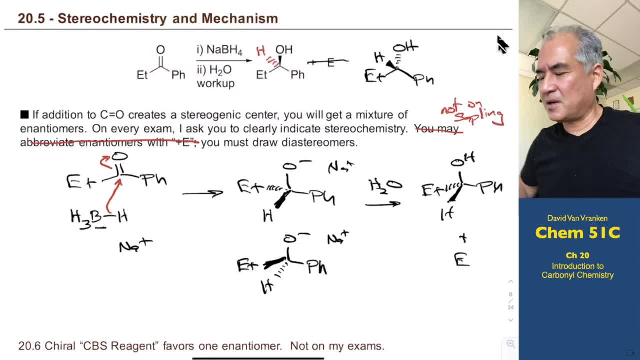 So on the sapling system, if you want to indicate that that there's an enantiomer, then you have to literally draw the mirror image or any other stereoisomer in order for the system to recognize that. So you can't say plus E. 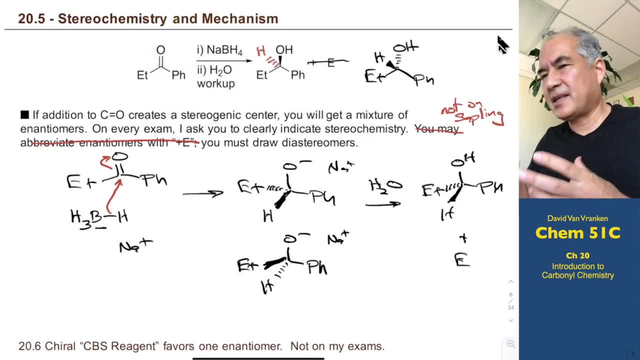 Okay, Which means I have to be careful about how I ask those questions, because I know it's time consuming. to draw a second enantiomer on your image of a molecule, There's a section in the book that talks about a type of reagent called a chiral reagent, called the CBS reagent. 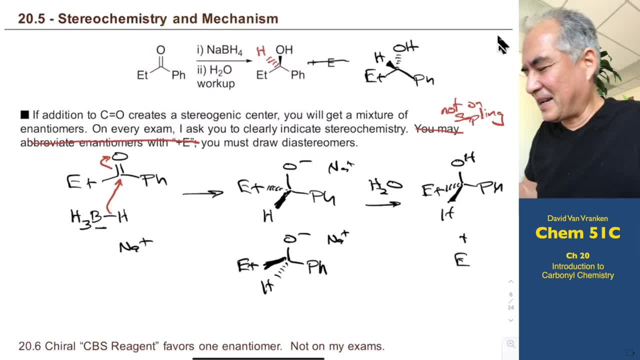 It's a- I'm forgetting that. it's Corey, but I forgot the name of the reagent- a borane compound with a um that has- that's chiral- that can choose and selectively add to one phase of a carbonyl rather than the other. 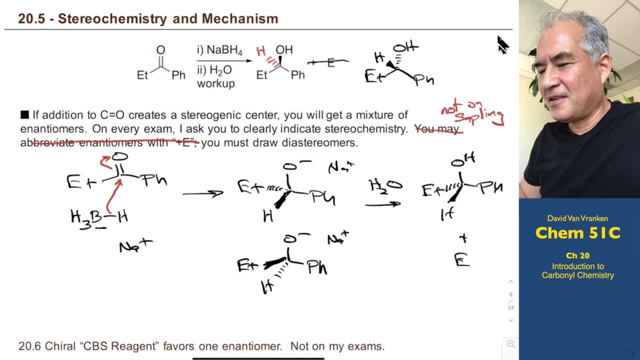 There is no reason in the world for you to memorize that reagent Um um. so I would prefer you just skip it. but you know you can read through it and it's interesting stuff for you to learn about, but there's no way I would ask you about that on the exam, because I don't think it's. 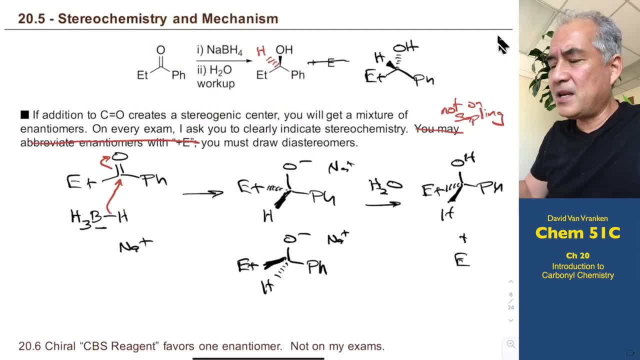 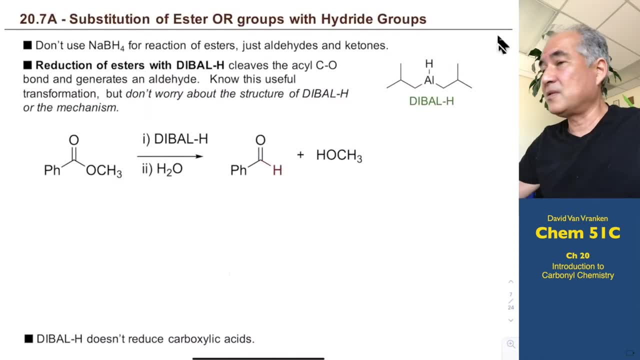 it's important for you to memorize that particular reagent, but be on the key view. be on the lookout for a formation of new stereogenic centers that weren't there before, because when that happens, you're going to generate a racemic mixture. 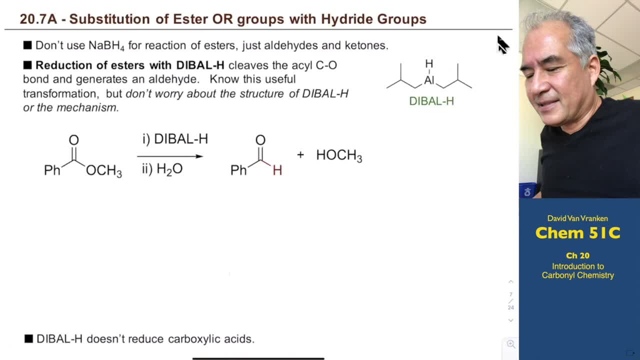 You have no control over that. All right, Okay, I just finished talking about ketones and aldehydes. You had a hydrido group in and it it's, and it forms a tetrahedral center where the carbonyl used to be. 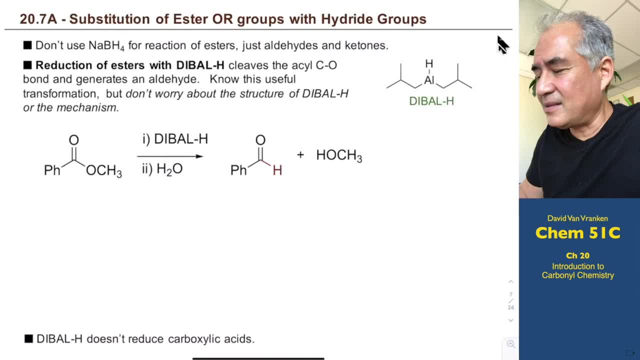 But I want to introduce you to an another reagent that doesn't really fit in here. It's not like lithium aluminum hydride, It's not like sodium borohydride, And you might say, Oh well, there's an aluminum in that reagent, and the reagent was called dibal H: diisobutyl aluminum hydride. 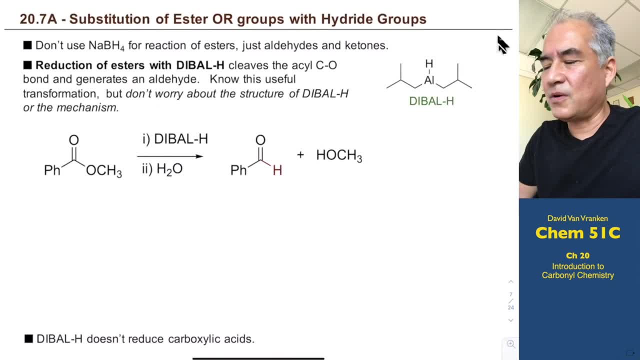 These four carbon alkyl groups are isobutyl groups. There's two of them, So it's diisobutyl aluminum with a hydrido group on there and dibal H. after this, you don't need to know the structure. 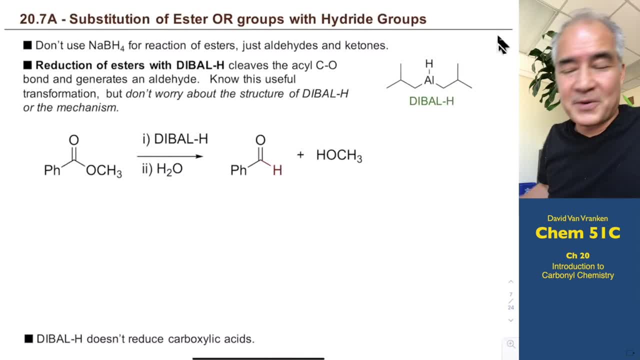 I'm never going to ask you the structure. The book doesn't show you The mechanism. So I'm not going to show you the mechanism because it'll. it'll freak your mind out if I show you the mechanism. But when you treat an ester, 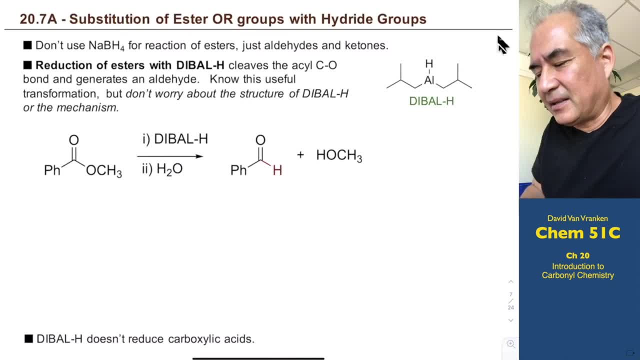 not a ketone or an aldehyde. if you treat an ester with dibal H, it replaces the ester alkoxy group with a hydrido group, and that is useful. Man, that's useful. Wow. Aldehydes are so much more useful than esters that, as far as the synthesis 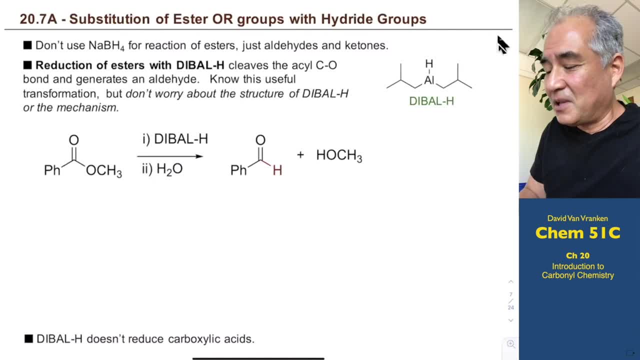 organic synthesis goes. So this is really an important transformation when when you do multi-step organic synthesis in the laboratory. So you need to know this two step procedure. You need an aqueous workup, just like we needed with lithium aluminum hydride. 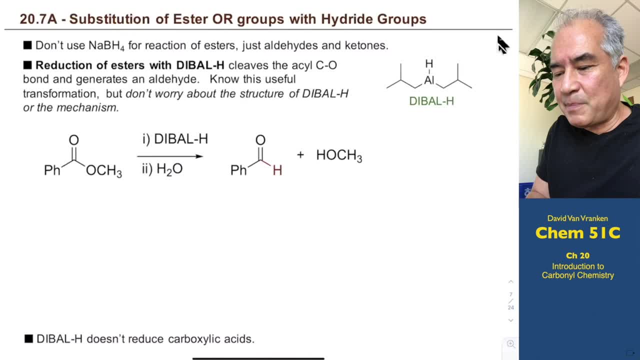 I'm not showing you the mechanism, but you need to know that any type of of ester bond like this is going to be substituted. It's going to be substituted. That bond right there is going to cleave and you're going to add the H group from the dibal H. 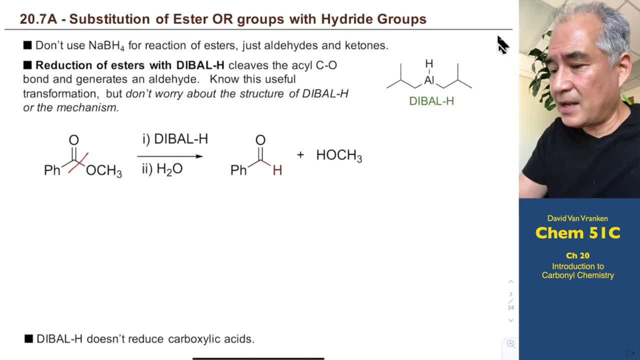 So it's super useful to turn esters into, into aldehydes, and it can be an ethyl ester, It can be a fennel ester, It can be a long 50 carbon chain on there, if you wanted, on the O? R part of the ester. 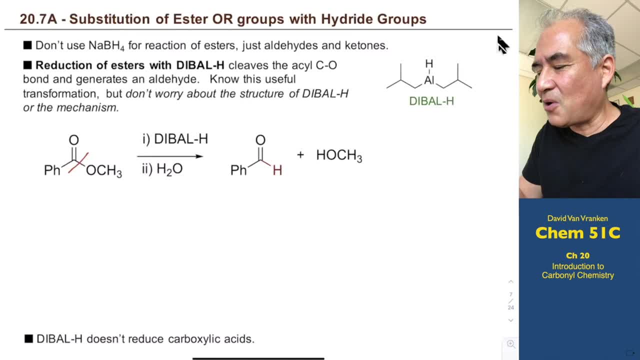 Doesn't matter. You're going to cleave that bond and make a new C H bond And normally you throw the alcohol part away. That's usually discarded as trash- almost always. So usually it's ethyl or methyl, because ethanol and methanol are easily evaporated. 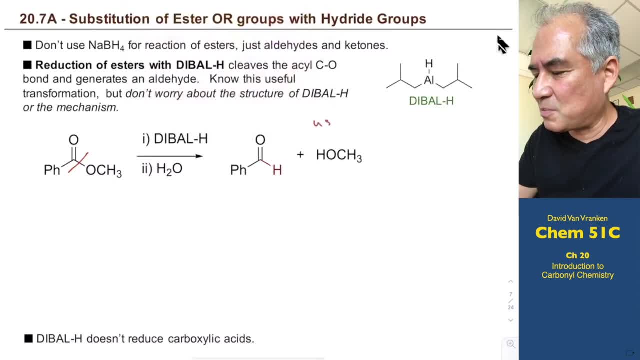 So I'll just write that this is usually the trash part Usually discarded. We usually just evaporate that off usually, So it's almost always methyl, but not always usually discarded. I think we'll cover later. in some of our problems It's cases where it's a cyclic ester and there's no way to discard it because it's the alcohol, leaving groups attached. 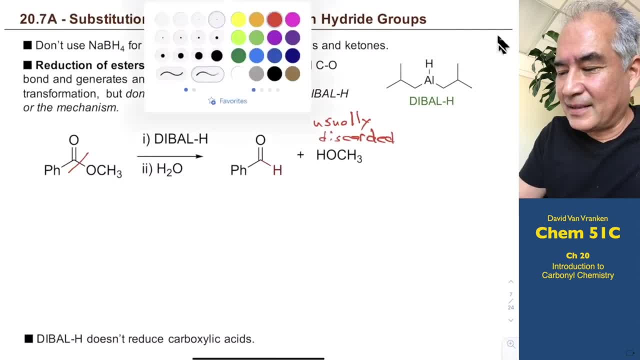 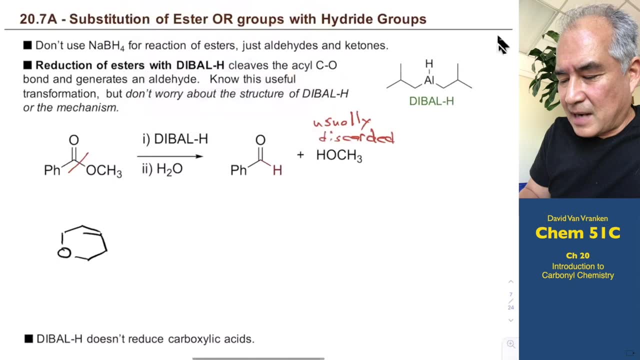 Let me go ahead and just draw an an exotic example to try to kind of stretch our minds here a little bit. and we'll try to make this super fancy. So I'll put an alkenes here, I'll take a pyrane ring. 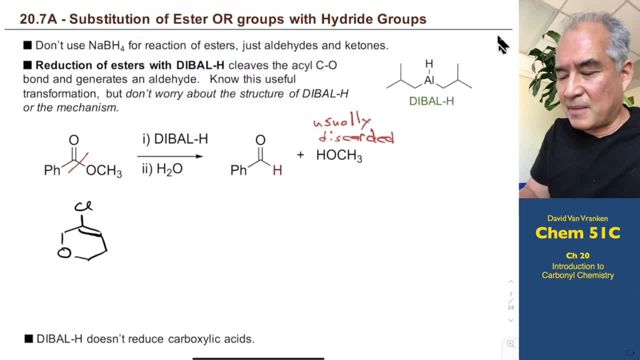 You don't know the name of that ring yet. I'll put a leaving group on the double bond. but of course you can't do SN2 or E or anything with that because it's on an SP2 centers. That's not going to react. 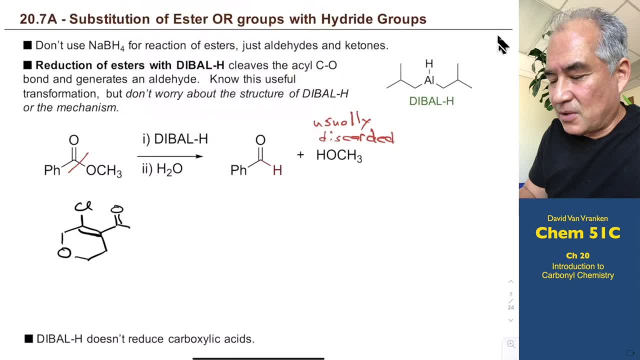 but I'll just dangle off on here and ester. So CO2, ET and ethyl ester would be a pretty common type of ester And if I wanted to reduce this down to an aldehyde so I could do some chemistry from. 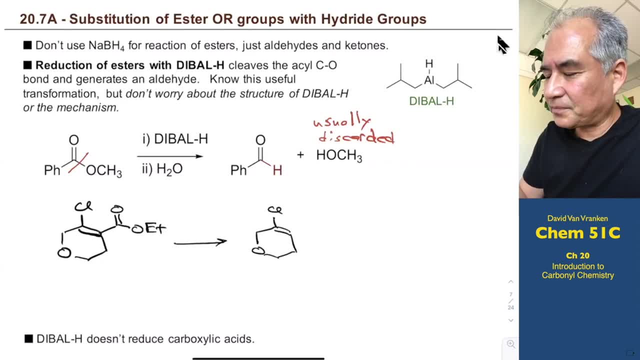 from chapter 21,, for example, which you haven't seen yet. let's just suppose I wanted to change that to an aldehyde. Right, There's an H on that aldehyde. I just didn't draw it Well again. 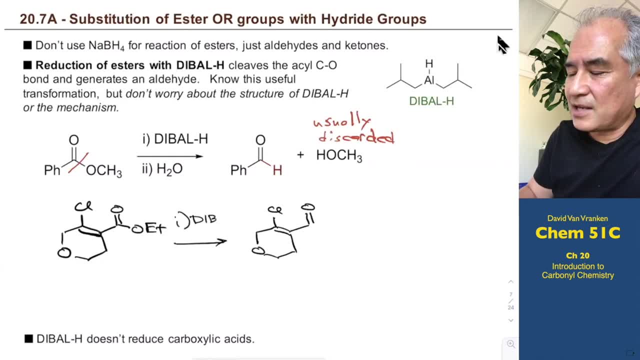 you use your DIBAL H reagent, DIBAL-H. and then step two, there's an aqueous workup, H2O workup. I can't resist writing the word workup because again, you're, you're kind of. 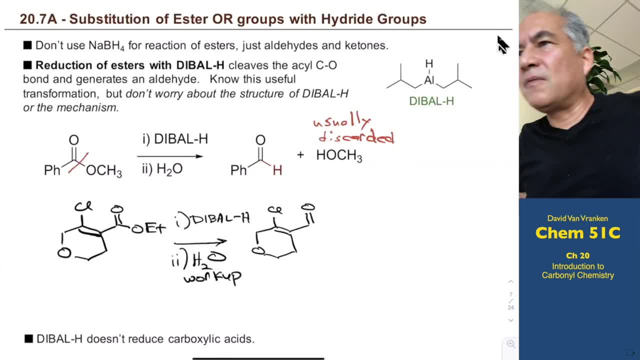 you should be getting used to this idea of of when you make alkoxide anines, working up those reactions by dumping in a bunch of water And you can't just write DIBAL-H. and you cannot write DIBAL-H and water and not enumerate the steps. 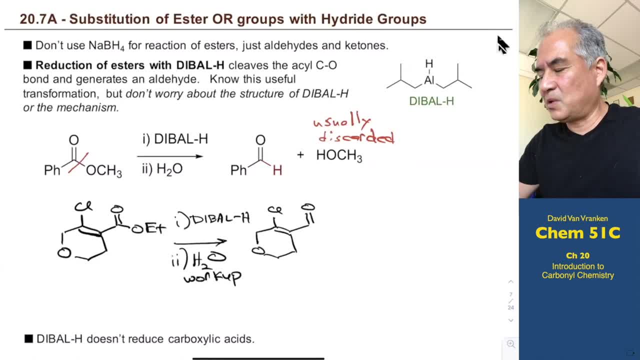 That's completely wrong. DIBAL-H would be destroyed by the water, just like lithium, aluminum hydride. So when I tell you to enumerate the steps, if you don't do that, that's wrong. So right If you have esters. 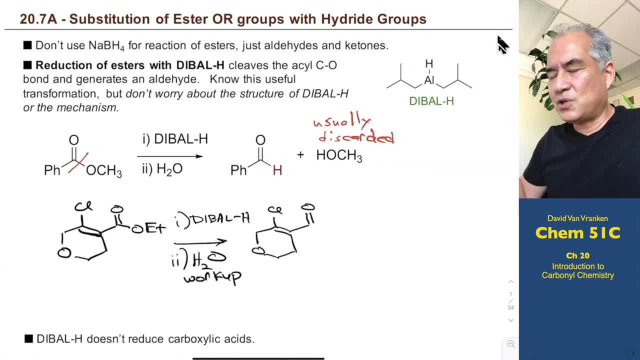 this is a powerful reaction. I'm sure somewhere in this quarter we're going to have examples where we do multi-step synthesis And one of the steps is reduction of an ester to an aldehyde using DIBAL-H- Remember that reagent. 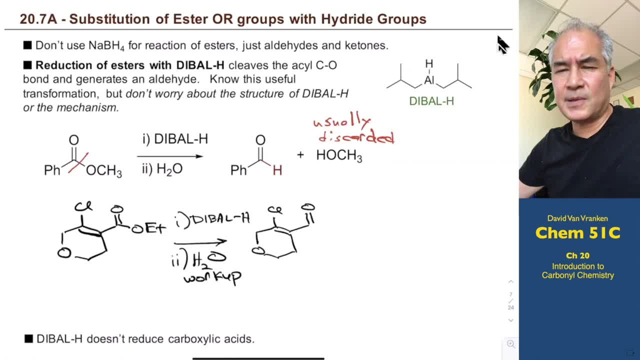 So not quite as common as lithium aluminum hydride or sodium borohydride, but super, but still super common and super useful. Okay, Let's go ahead and take a look at another reaction of esters that uses lithium aluminum hydride. 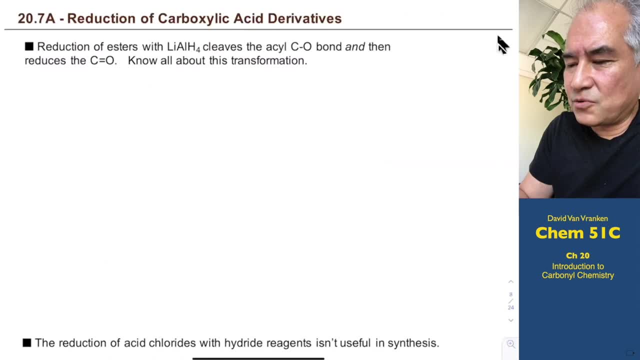 Okay, So let me go ahead and draw out an uncommon, or maybe let me go ahead and try to draw out something that looks a little bit fancier than just a regular ester. So this ester has a double bond attached to it. 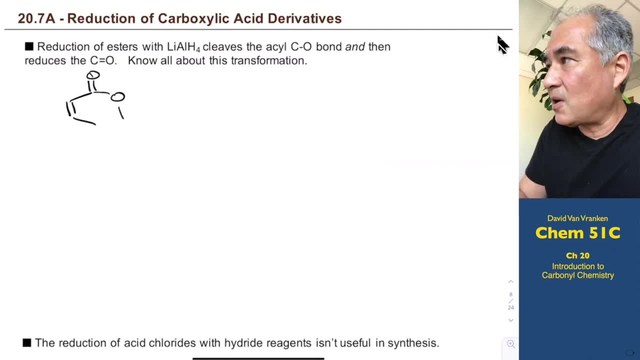 So if we wanted to reduce this all the way to the alcohol- and you have to watch this pattern of reactivity here- then we use lithium aluminum hydride, And let me show you how this works. Okay, So we have a double bond attached to it. 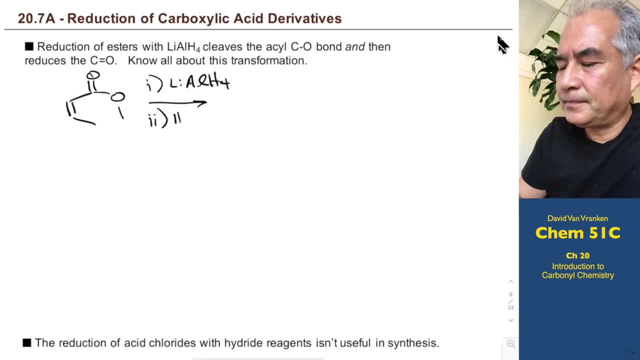 So we have to follow this up with an aqueous workup And the product of this reaction still has this cis double bond on here, but it reduces the carbonyl group all the way down to an alcohol And it cleaves this bond here. 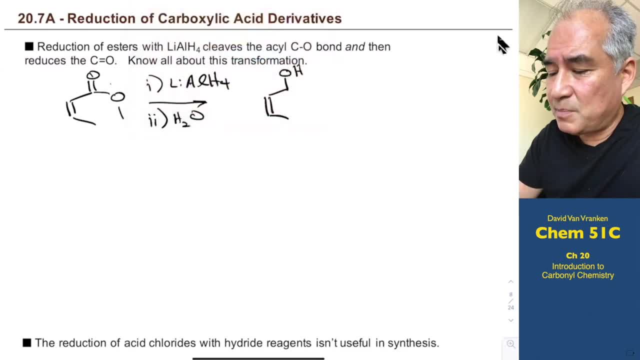 Let me go ahead and draw the bond that gets cleaved, And it cleaves this bond just like the DIBAL-H did. So you end up with, as a byproduct, this methanol as a byproduct in that, And this is the process. 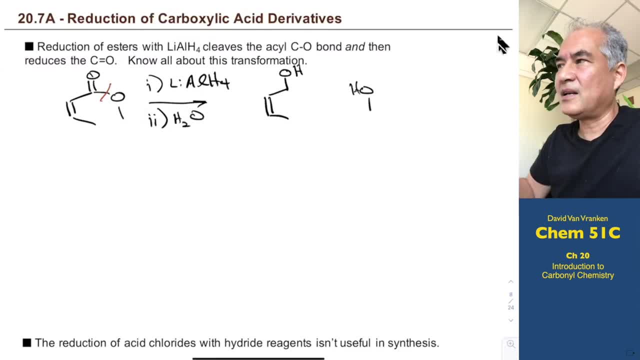 So if it was an ethyl ester, you would end up with ethanol as a byproduct. And usually you do this with a methyl or ethyl ester because you're usually trying to evaporate away the methanol or ethanol. That's typical. 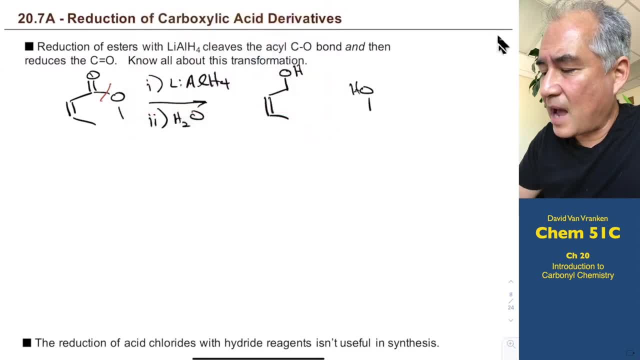 So what am I not showing you here? What I'm not indicating that just happened is we added two equivalents. We added two hydrido groups to this, So lithium aluminum hydride actually carries four hydrido groups and it can transfer all four of those in there. 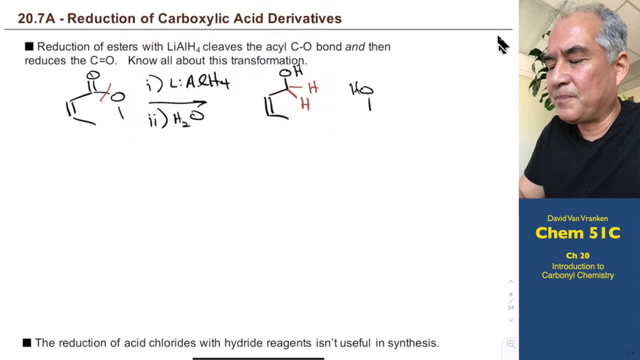 Actually I'm not writing down stoichiometry here, but one equivalent of lithium aluminum hydride would be enough to reduce two or one mole of lithium aluminum hydride would be enough to transfer hydrido groups to two equivalents of the ester. 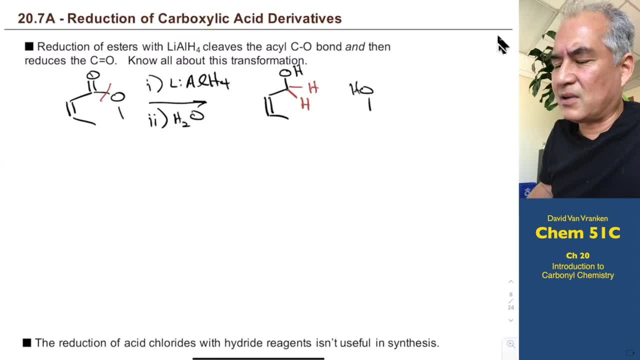 And so I'm not worried about in this particular case. you just have to assume that it's when we're doing these reductions of esters with lithium, aluminum hydride that you're adjusting the stoichiometry. So the book shows you that you can take other types of. 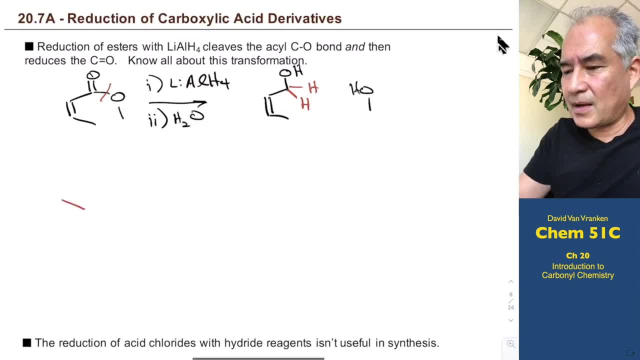 even more reactive ester carboxylic acid type derivatives, like acid chlorides, and do this same type of reaction. So I can have an even better leaving group than a methanol or a methoxide leaving group and do this same process. 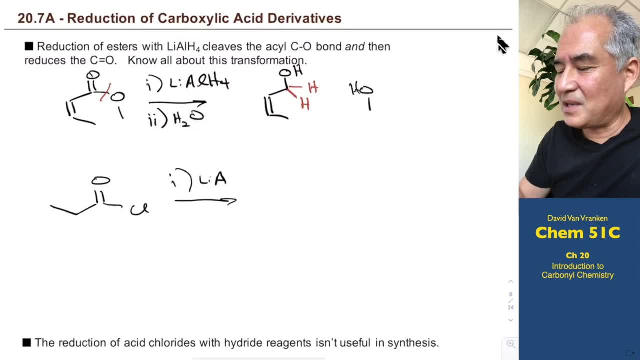 Honestly, nobody would ever do this, but if you did, it would certainly work even better. We'll talk more when we get to chapter 22 about the reaction activity of various different acid chlorides versus esters versus carboxylic acids. 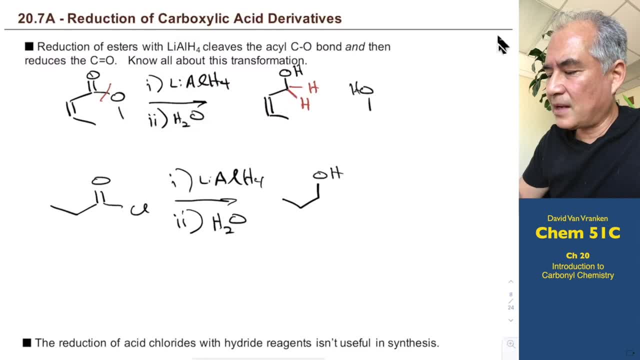 So you can do the same type of reduction here. And in this case I'm not going to draw the chloride. We normally don't draw the lithium salts or the chloride salts as the product. We just show the organic products of the reaction. 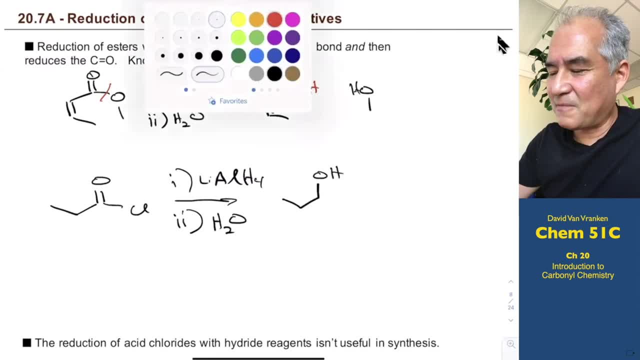 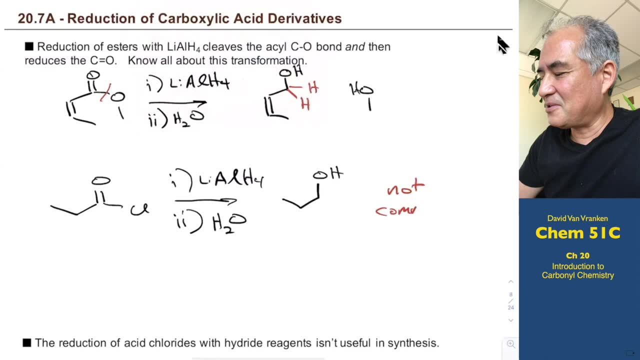 This is just. nobody would ever do this. It takes a lot of work to synthesize acid chlorides. If you go through the trouble of synthesizing an acid chloride, there's no way you're going to take it and reduce it. You're going to reduce it right back down to an alcohol. 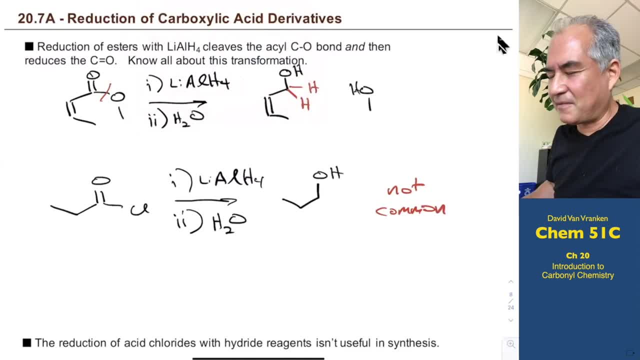 It's just. this would not be in any way common. I can't envision ever asking you this, because nobody would ever do this. It's not a useful process in synthesis, But the book seems to ask a lot about this and you might get asked that question later on some sort of MCAT exam. 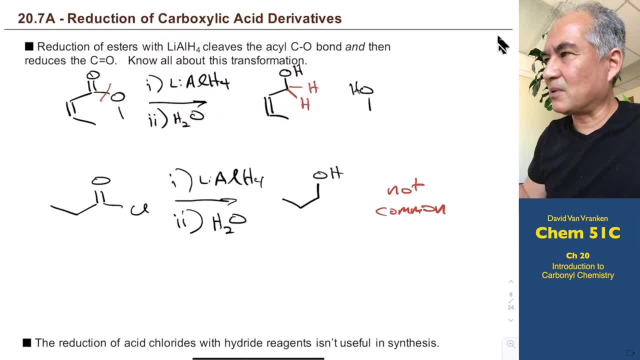 or graduate record exam to get to graduate school or something, But nobody would really do that. It's an academic exercise. Wow, What's happening here is the hydridoilluminate is adding to the carbonyl group. We'll talk about this mechanism here. 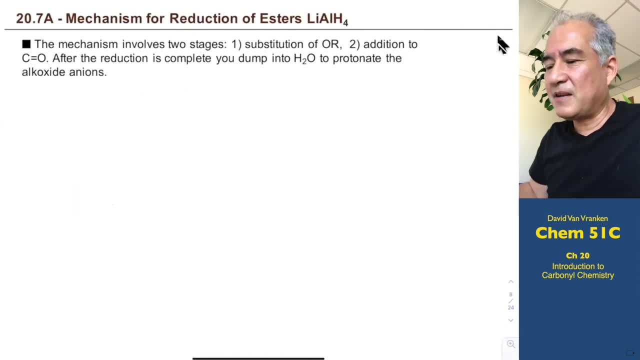 It's an important mechanism and it'll help reinforce this idea that when you see a carbonyl, add nucleophiles to the carbonyl. Let's take an example of ester reduction. What's going on mechanistically when we add to an ester? 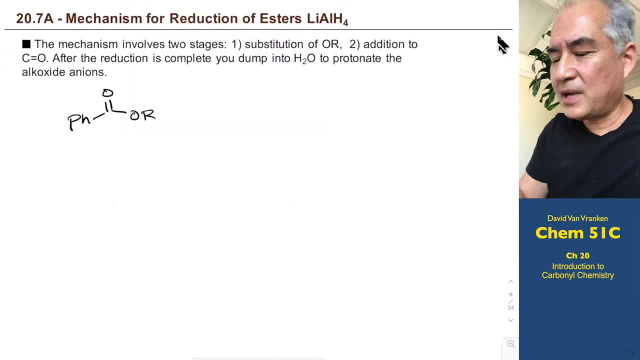 We'll make this an ester of benzoic acid. Who cares what the R group is? It could be methyl or ethyl, Those are typical. And when we add a hydridoilluminate reagent in there- lithium, aluminum hydride. 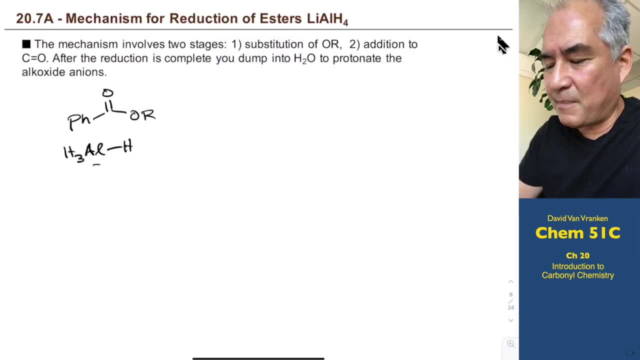 that long nucleophilic hydridoilluminate bond is going to add to the carbonyl. The hydrogen is going to form a bond to the carbon. So like this, Let me use my fancy red pen here- There we go, And so you form a bond to the carbon using that hydrogen atom. 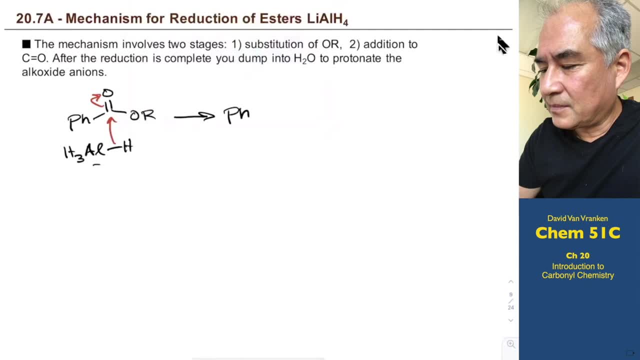 that nucleophilic hydrido group. Now, as soon as we do this, boy, this is going to freak you out. Oh my gosh, This is probably going to be the wildest thing you've ever seen. We're going to generate this intermediate where there's this nucleophilic O minus. 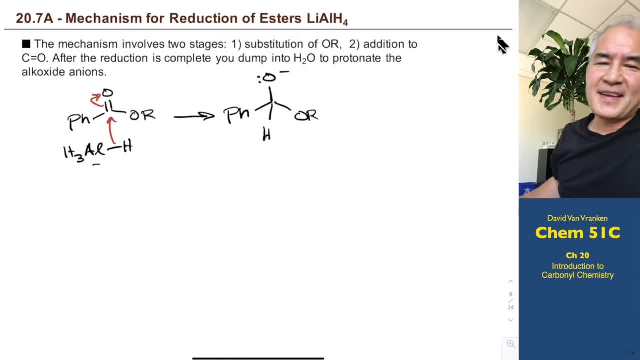 And right next door there's an alkoxide And that alkoxide is going to act as a leaving group. Now, probably somewhere in the organic chemistry series, you were told: oh, alkoxides never act as leaving groups. And I said two reactions. 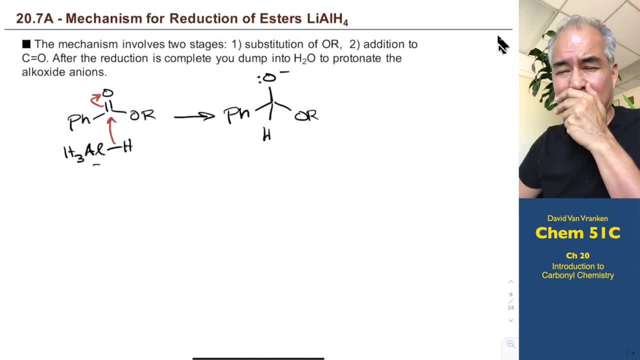 Yeah, Oh yeah, There's a leaving group in an SN2 reaction. That's SN2 reactions. Alkoxides are not leaving groups in SN2 reactions And hydroxide is not a leaving group in SN2 reactions, But this is not an SN2 reaction. 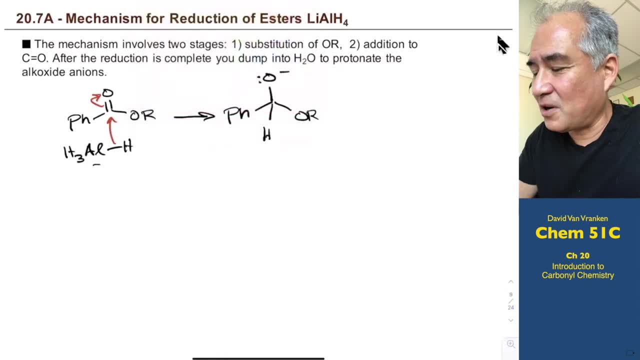 The nucleophile here. the O minus lone pair, which is a strongly nucleophilic lone pair, is right next door to this carbon atom. See that carbon atom, This O minus, is right next door and cannot ever get away. It's always pushing. 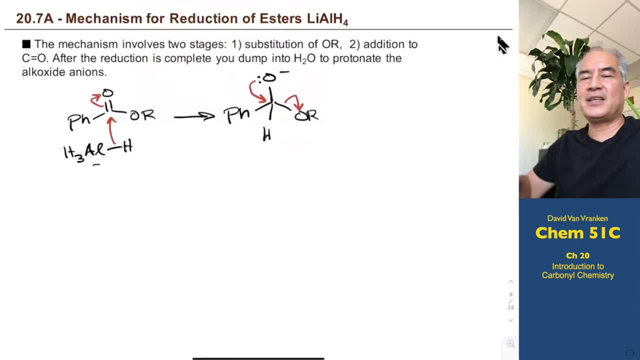 always pushing. So there is absolutely no problem pushing out the alkoxide anion as a leaving group. So when we talk about these intermediates that result from addition to esters or carboxylic acid derivatives, there is absolutely no problem pushing out an alkoxide anion. 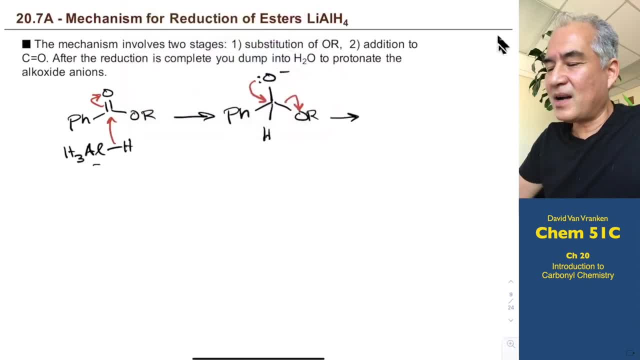 So if you thought you memorized that alkoxide couldn't act as a leaving group, that's only an SN2 that they were talking about, No problem. We're going to see this over and over and over again in this quarter, where alkoxide anions act as leaving groups. 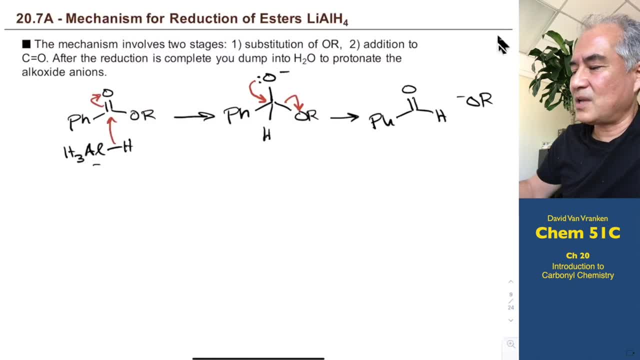 and hydroxide in some cases, depending on what the substrate is. So this might not be part of your normal repertoire of leaving groups that you're used to seeing. Now notice: we've generated an aldehyde, And aldehydes react with tetrahydroilluminate. 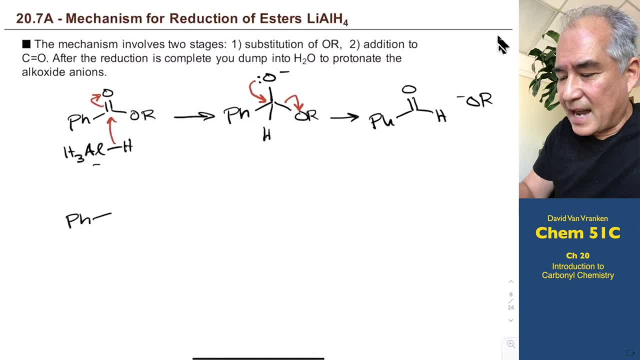 So if you've got extra tetrahydroilluminate, or if we kept count here, there's actually more than one hydridoilluminate bond on our starting material. I'm just going to draw this with. I'll just go ahead and draw this. 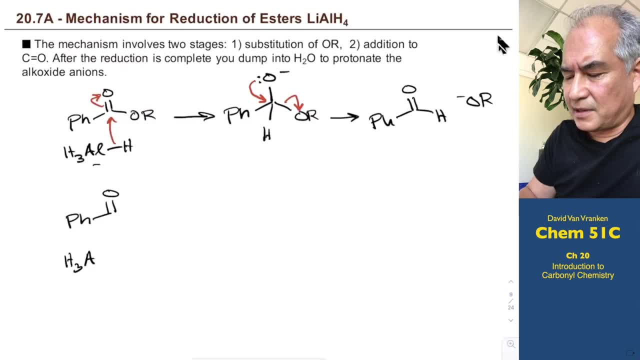 with another equivalent of the tetrahydroilluminate. But there's other species in there floating around that have these nucleophilic bonds And this is the way I would encourage you to draw the mechanism, because who cares what the other three things are in this aluminum? 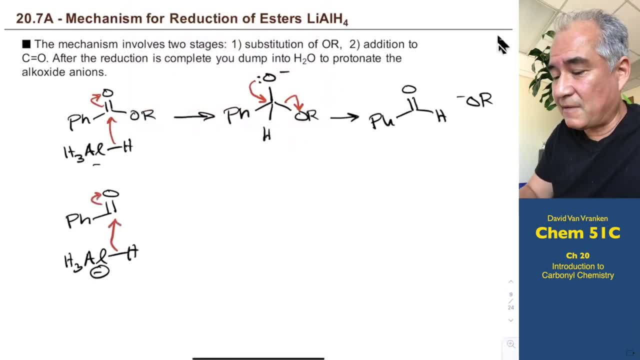 There we go. So as soon as you generate that aldehyde, even faster than the original starting material, you can't stop this at this point. You can't stop it. The other molecules of tetrahydroilluminate, the second, you generate an aldehyde. 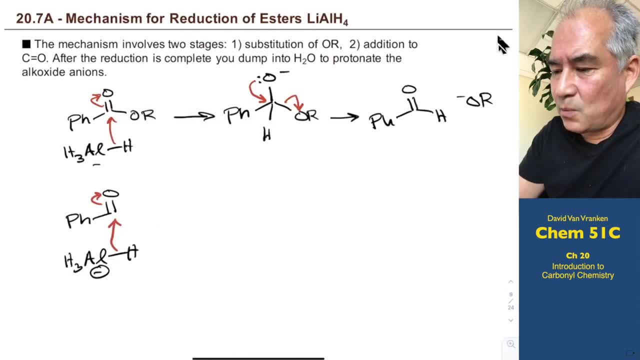 will react even faster with this aldehyde than they react with the ester, And so you'll end up adding a second time, And that generates this alkoxide product. Let me draw the H that was there before. Now we've got two Hs. 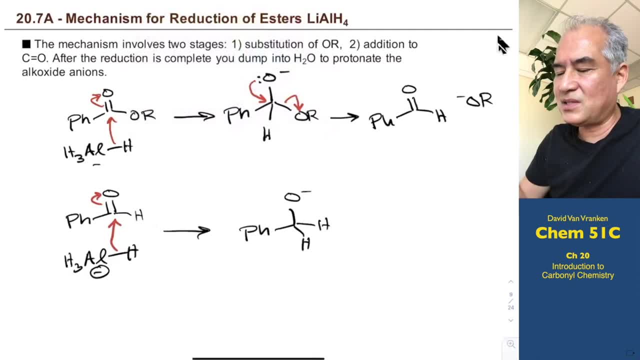 And this is the product that results at the end of this reaction. It's going to be sitting in there with your lithium salt floating around, Li+. If you had an Li plus counter ion here, associated with the lithium aluminum hydride, So that'll just sit there and sit there, and sit there. 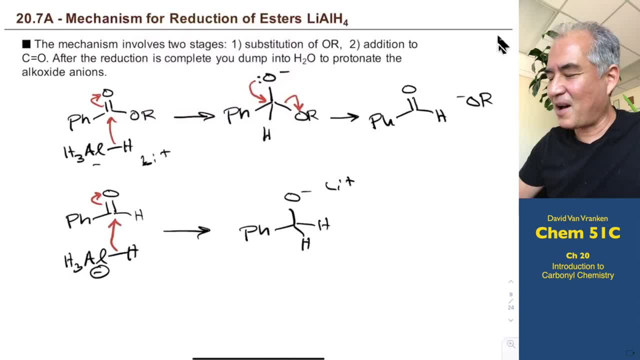 You can come back three days later. but you need to come back if you want to isolate your product and work this up, Convert it to something neutral by dumping a bunch of water in there, so that now you can extract it into an organic solvent and then just evaporate the solvent. 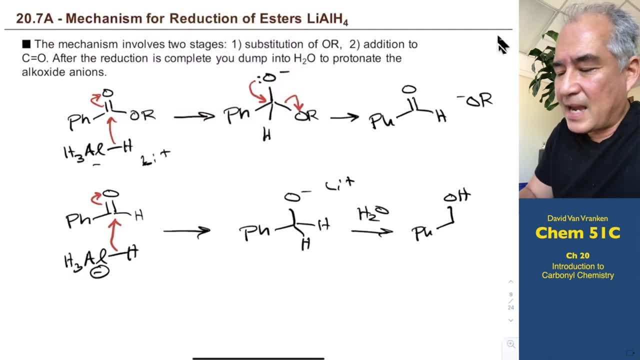 and you've created benzyl alcohol. So look what we've done. If you take an ester, through two additions to the carbonyl group- get used to adding to carbonyl groups- we can convert esters to alcohols. 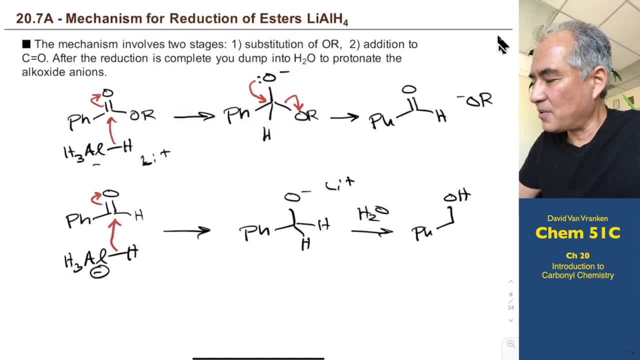 Now, what happened to this OR minus group? Well, that's also there. It's usually ethanol or methanol, And so that usually just gets evaporated off along with any solvents that you use for the extraction. It would be rare that you would care about the OR group. 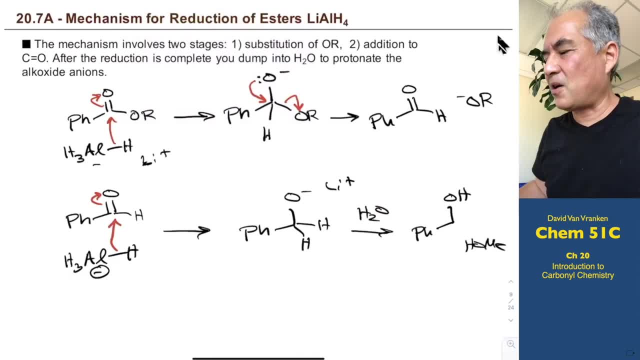 Maybe if the OR group was some big heavy molecule that you couldn't evaporate off, You'd have to worry about that. So there's actually two products here. If I asked you to draw the products of the reaction, the products I'd expect you to draw: the methanol. 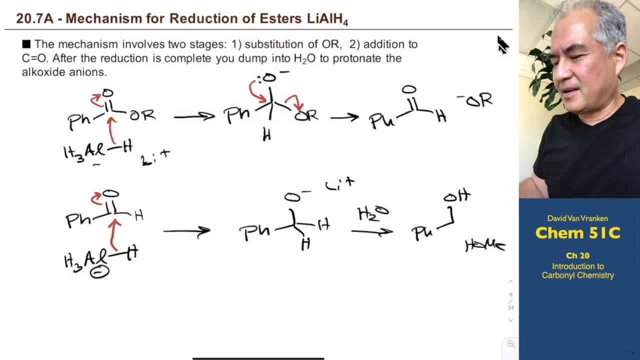 but really we usually like to reduce esters with methyl or ethyl esters, because then we can just evaporate that part off. All right, I'm going to go ahead and stop right there. We've made some decent headway here, And when we come back? 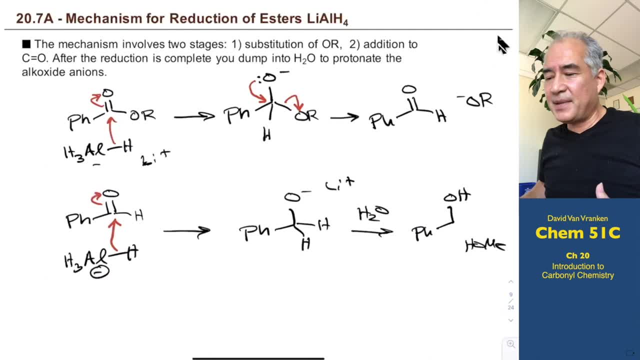 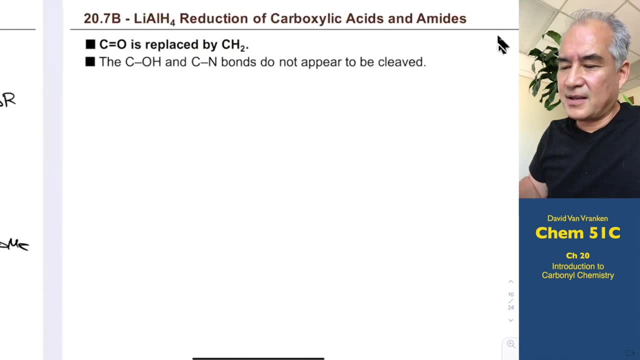 on, I think, Friday we're going to talk about reduction of amides And the really key thing that we're going to get to- let me see how far off I am from that- is addition of carbon nucleophiles to carbonyl groups. 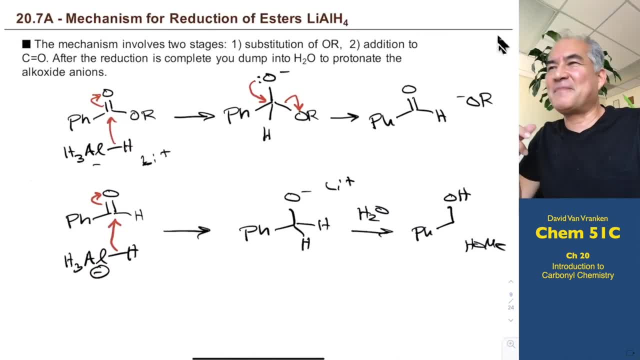 And that's really the meat of this chapter- is forming carbon-carbon bonds. If you're an organic chemist, like me, you love to form carbon-carbon bonds. Everybody who teaches in the organic chemistry series here at UC Irvine loves to form carbon-carbon bonds.